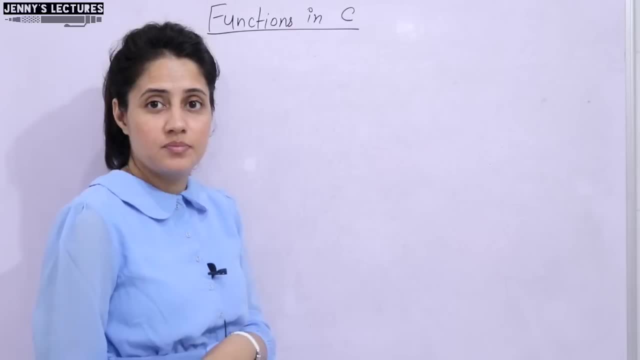 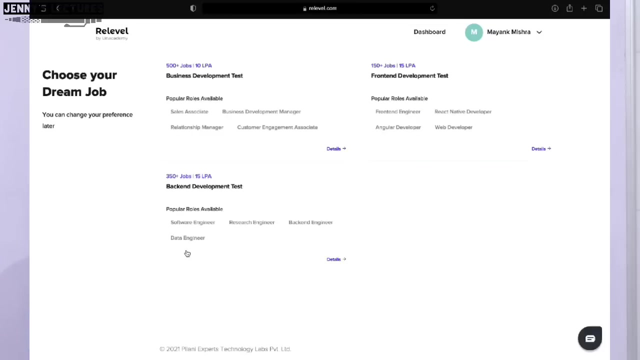 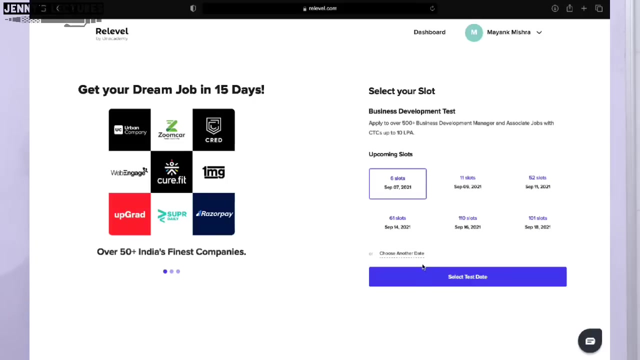 goal, Although you have applied to many companies. So here relevel is going to help you. It would be very beneficial for you. Relevel is India's first test hiring platform by an academy, which is helping job seekers find their dream jobs. It's very simple: You just have to sign up on relevelcom. Select the test of your choice: business development or front end development and back end development. Book a slot when you want to take this relevel test, Create a good and neat video resume and just click submit. 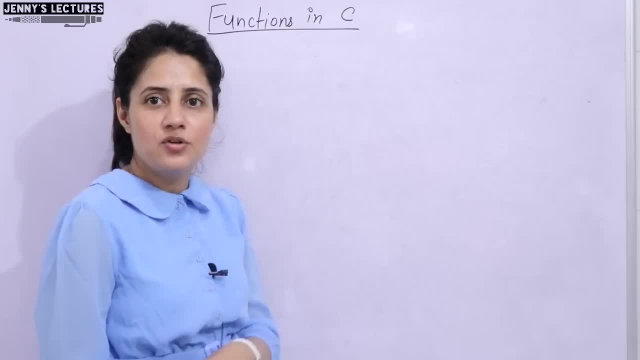 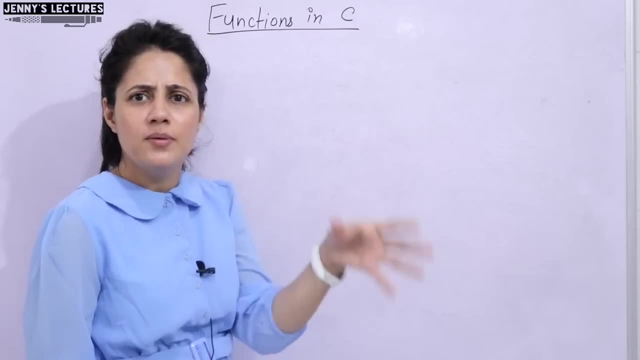 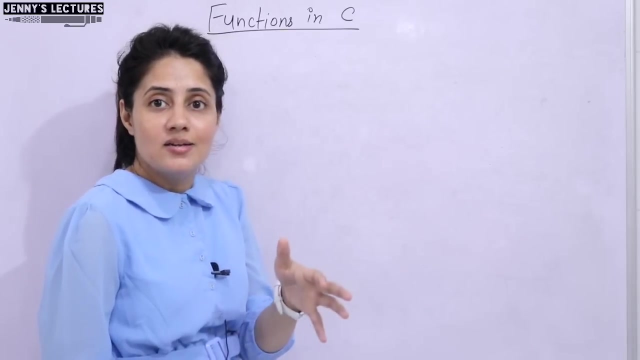 And confirm your slot for the test. So what is the benefit of this thing? See, over 50 plus companies, including top startups and unicorns like grad upgrade and urban company, and many more, are hiring through relevel. Here you will get 1000 plus job opportunities across business development, front end development and back end development. The best part is you can take this test for free, So you just finish your test in a single day and you will get your relevel score within a week. And once you have cleared this test with qualified 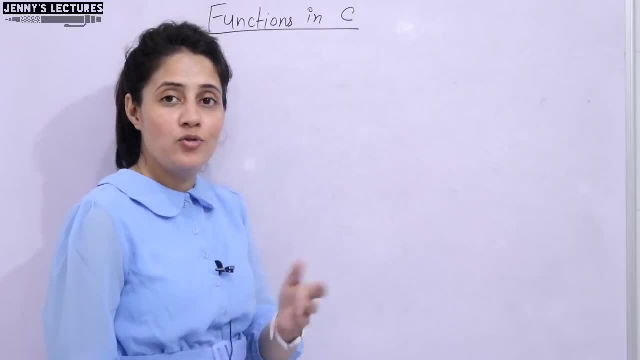 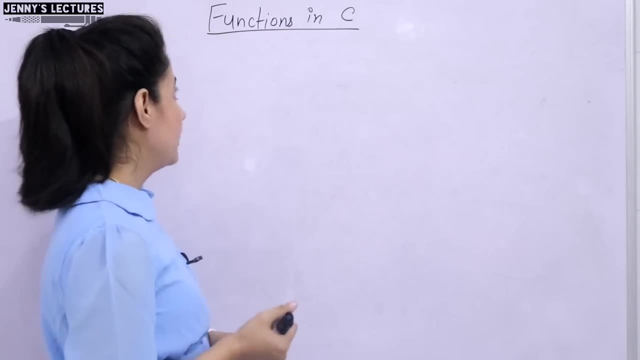 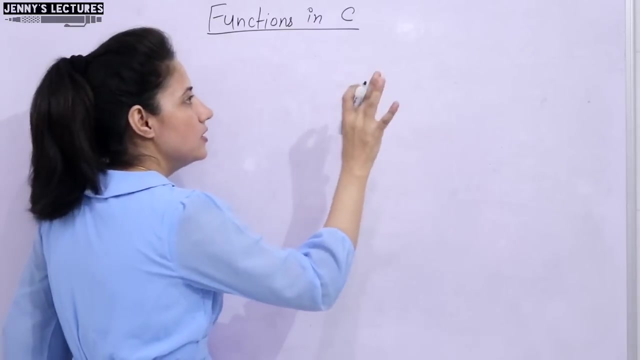 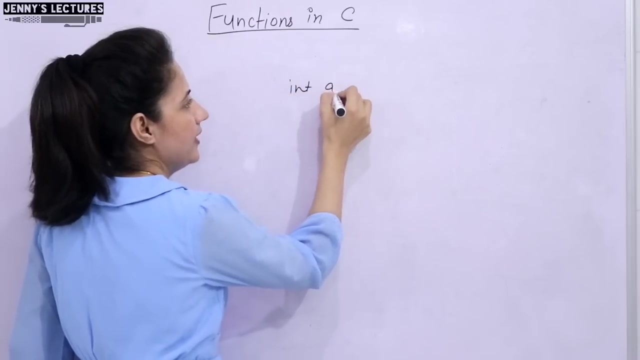 score. now you are able to create an amazing candidate profile. So while you are waiting, just register for this. The registration link I'll put in the description box of this video. You can go and check out. So now back to the topic. functions in C- See. before going to the actual definition, let me just take one simple example. Suppose a simple example I'm taking. I want to do sum of two numbers. So what you will do, we will take two numbers and one will take sum In sum is equal to: I'm assigning 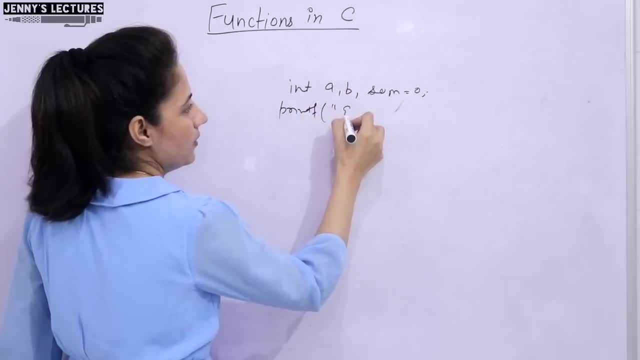 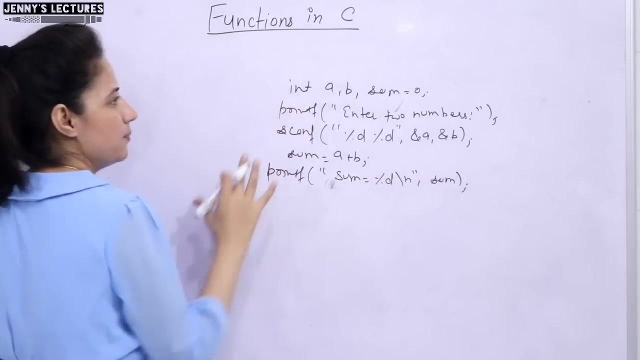 a zero. I'm initializing it with zero. Using printf, I'm writing: enter two numbers. I think you can easily write down a program to add two numbers. So this is I guess a simple program to write down sum of two numbers and here simply suppose you are writing it in here. 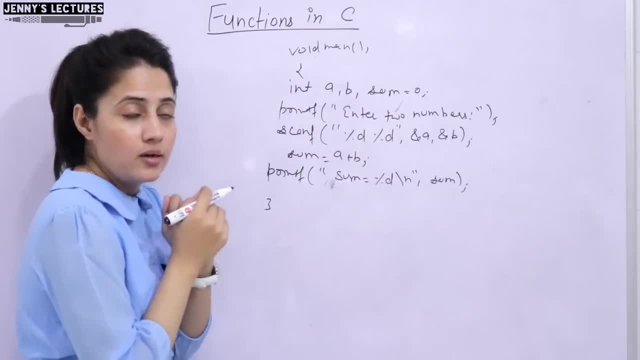 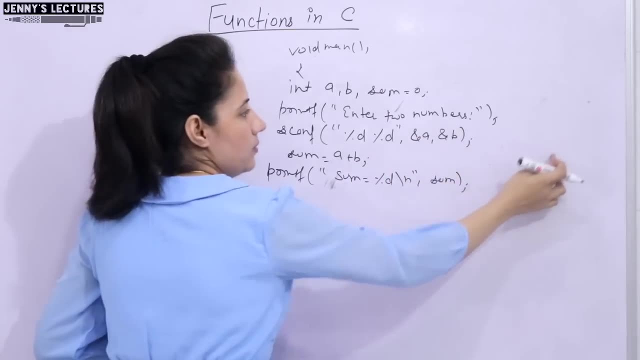 main function: header files and that's it. But here situation is: if you run this program, it will give you what output you will get. Enter two numbers. you will enter two number and it will give you sum One time. it will give you sum, You will run it one time and 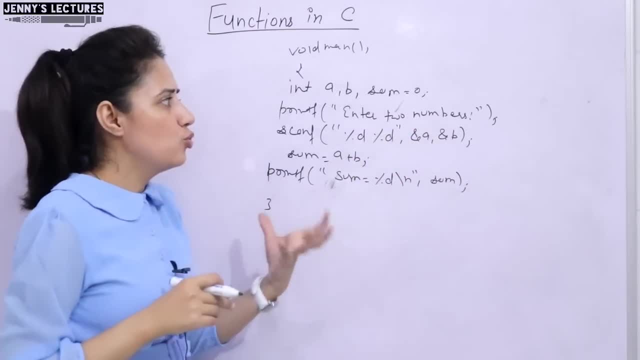 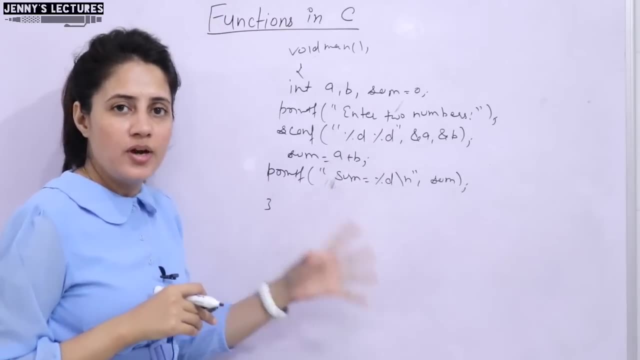 it will give you run sum one time. But here suppose some situation is like that: In a program I want to, you know, calculate sum. I want to sum two numbers multiple times, five times, six times, seven times. Right, So what you have to do If you want to do, 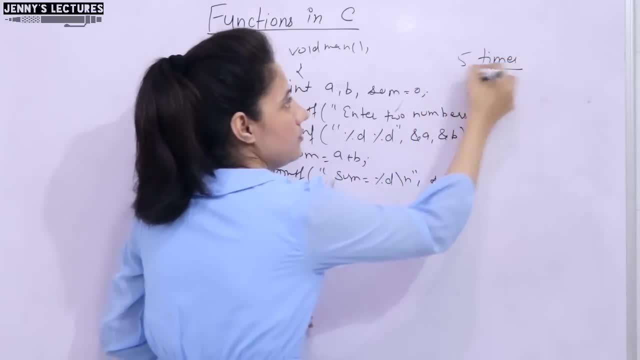 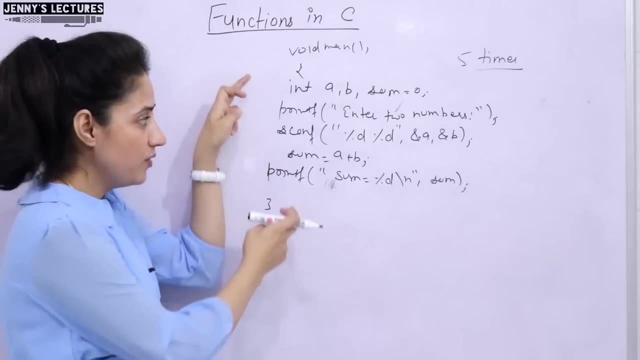 sum of two number five times in your program, Then five times you will have to write down this code, Right? Because if you run this one time it will give you sum one time. So if you want some five time, you will have. 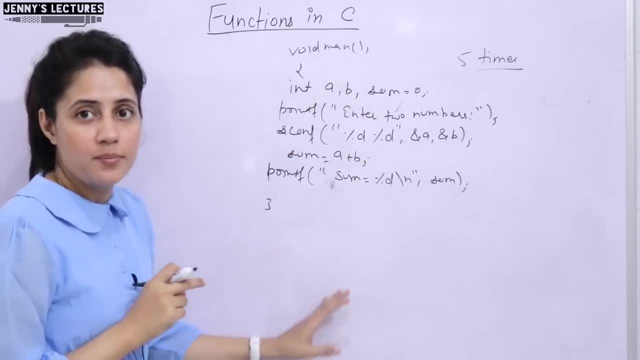 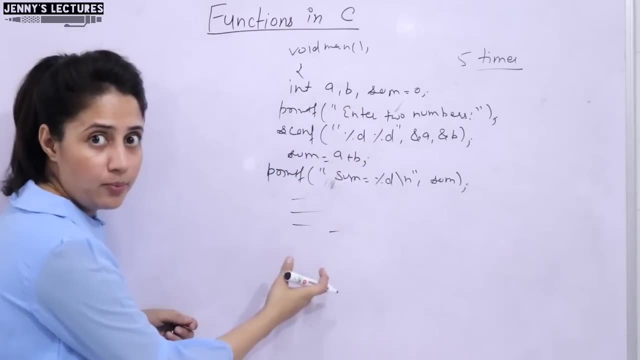 to run sum you will have to write down this code, some of this, the numbers five times in your program. Suppose, here I'm writing sum, after that I'm doing something in I'm in my program. again I want to do sum of two numbers. Again I have written some lines of. 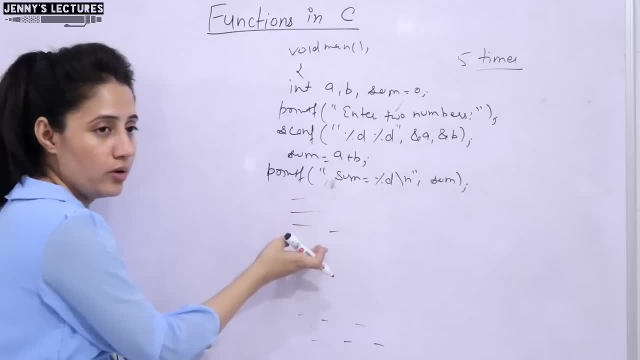 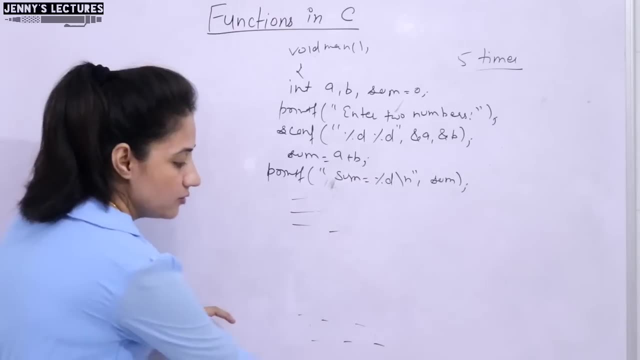 code. I want to do some other task, or maybe I want to here. I want to, you know, get some calculate. I want to do subtraction of two numbers. that thing is also possible right again, five times in your program. I want to do sum. so if you write down these lines again and 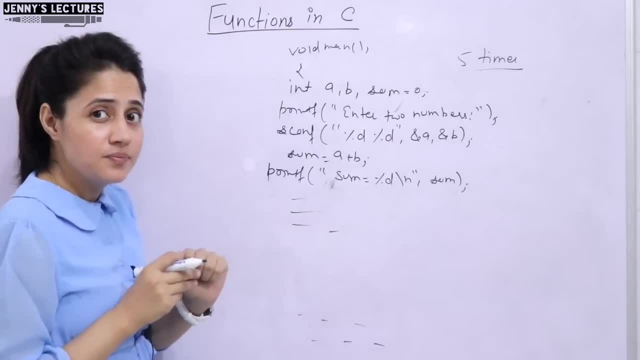 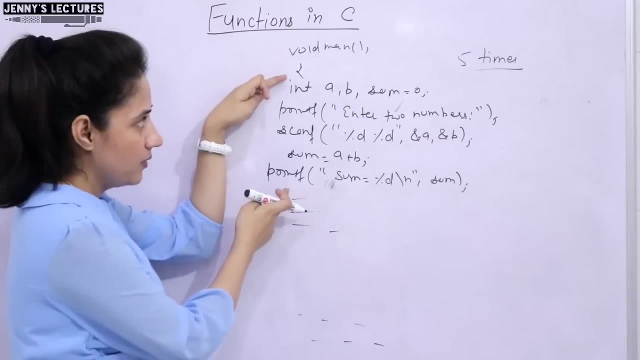 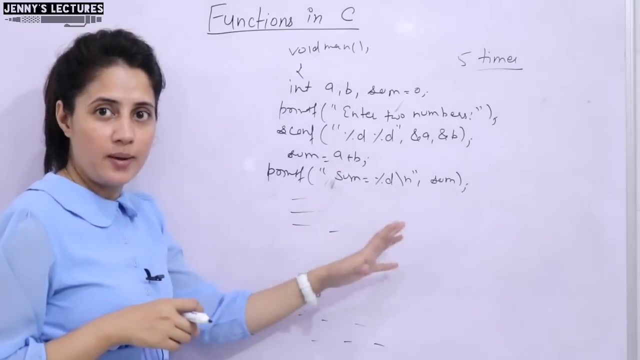 again five times? definitely your program would be lengthy. yes, I don't want to write down these lines five times. is it possible to write down these lines only one time and five times? I get sum in a single program in my program? yes, it is possible. how, using functions, suppose? 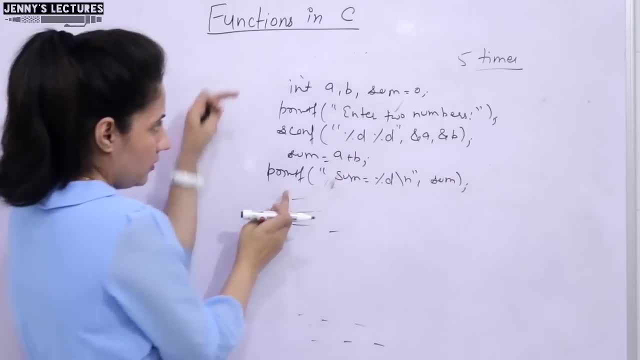 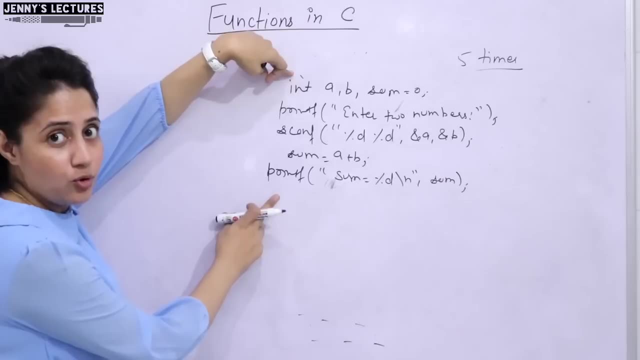 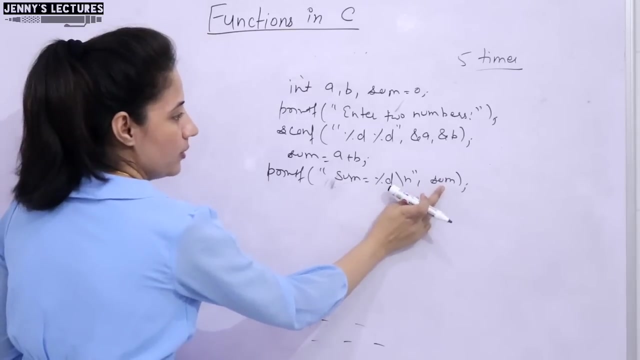 I do this thing. these are the lines which are required to do sum of you know. this is the code you can say. or you can say: these are the statements which are necessary. you have to write down these statements to write to you know: do sum of two numbers, so what you can do. 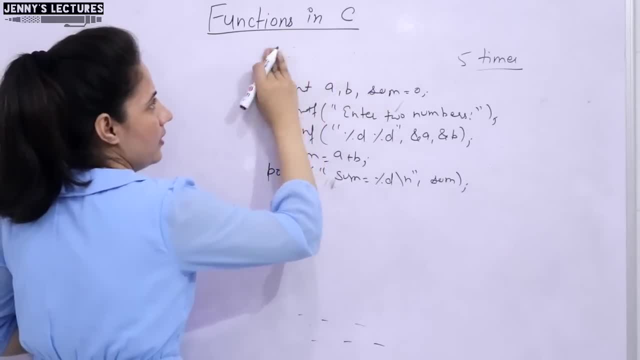 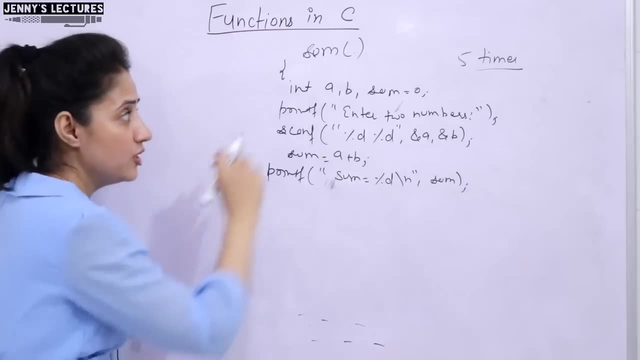 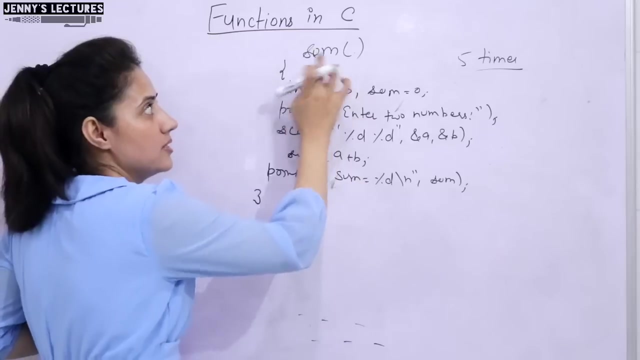 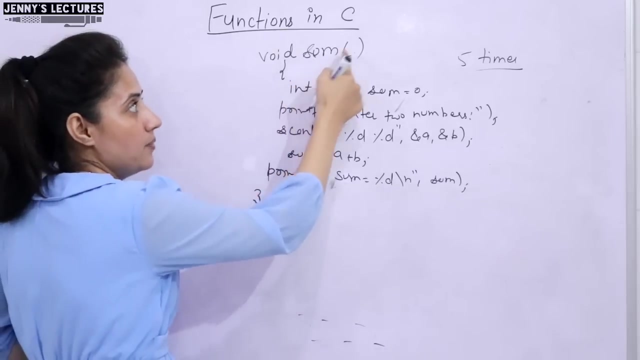 I can name this thing. suppose I can. I am naming this like sum. just put these lines into this curly braces and name this. I am writing name sum here, right, and return type. also. suppose I am writing void, void sum. if you write down something like this- these braces, these brackets, this is what function, you can say so now. 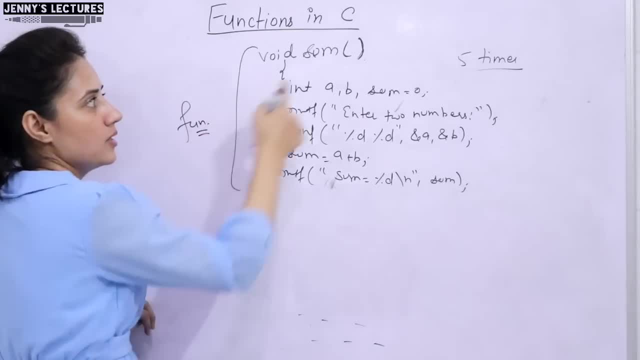 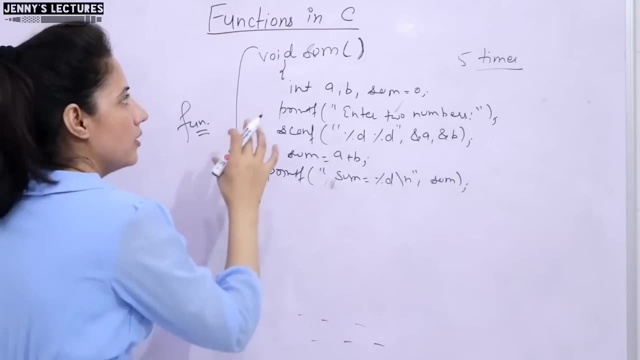 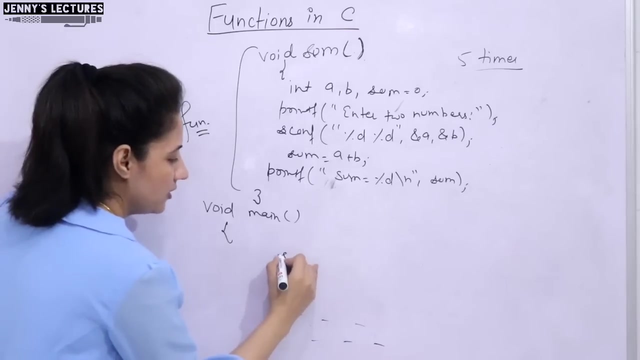 this becomes the function of the program. sum is a function. you can say: this is the function and name is sum. now how to, how to calculate, how to do sum five times in a program. now in main function, I am writing main here, right in main function. I am calling this one sum, that's it. 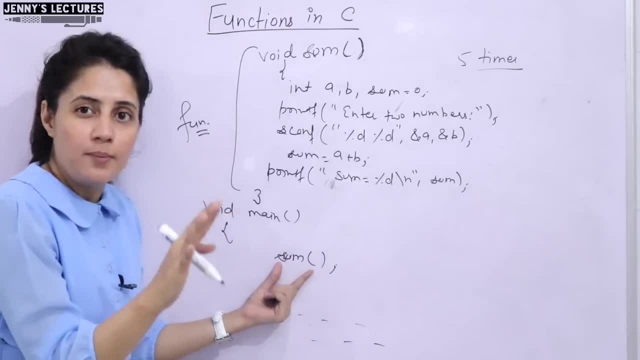 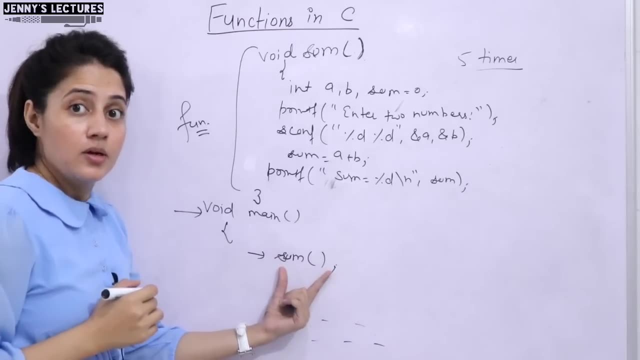 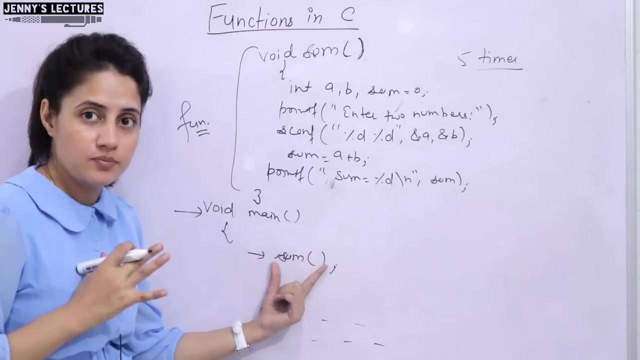 so obviously when you run a program directly, first of all control, go to main function. the first line is sum. now we know sum is what compiler has to do. sum of two numbers, sum of numbers, maybe two or three, how many numbers, we don't know. but you have to tell compiler properly like how to do Sum compiler has, compiler is: 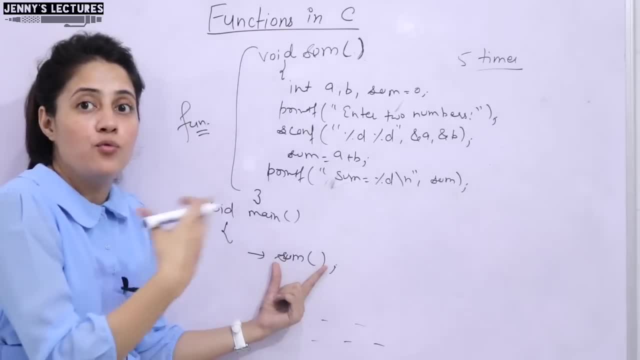 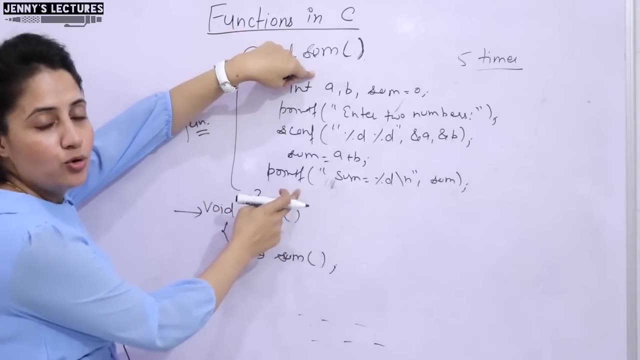 not having its own mind. so you have to tell. and where you are telling. here you are telling that you have to calculate sum. this is the method. or you can say: this is the process. this is the process to do sum of two numbers, right. So now this is. you can say: 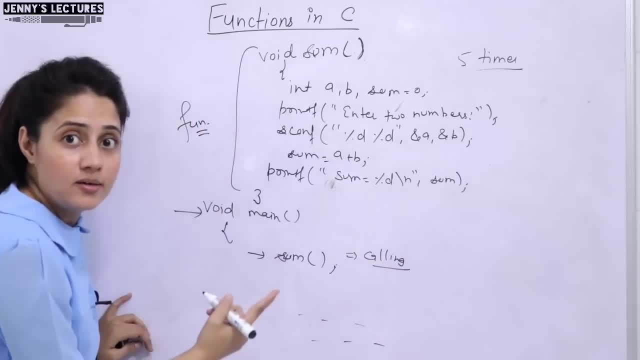 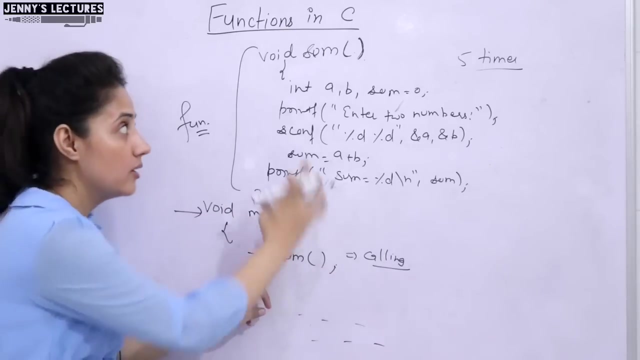 we are calling. we are calling the function sum. So whenever compiler will see this thing, this is what calling of a function, So it will search where this function has been defined, where the meaning of this function has been written. here we have the meaning, So control. 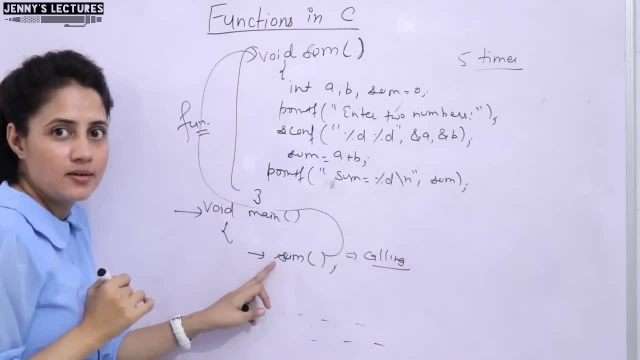 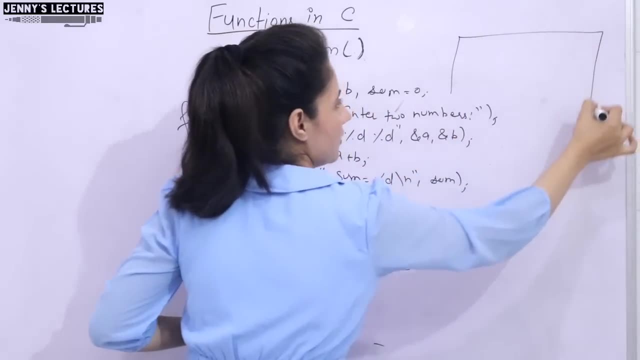 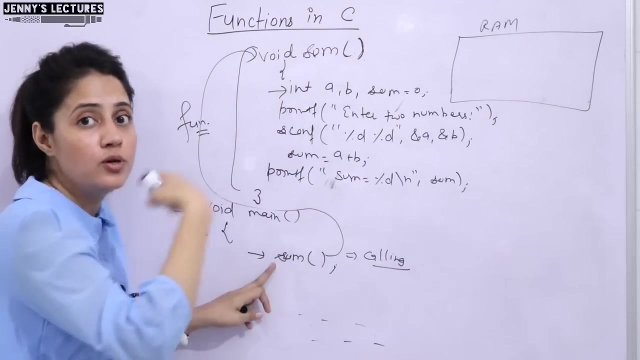 will go to here directly and now first line this So now in memory, in memory. what would be done? this is suppose a RAM, main memory. So whenever we run a program, definitely first of all it would be loaded to obviously main memory RAM, right? So main main would be loaded here. 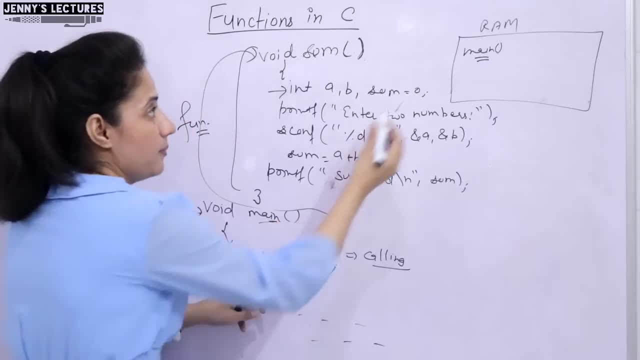 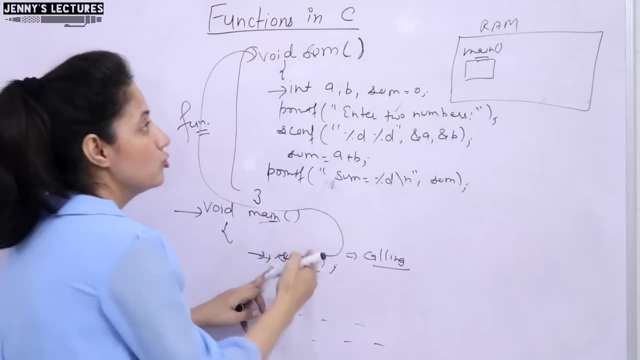 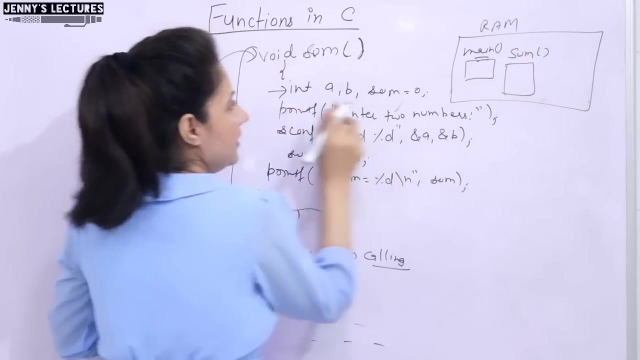 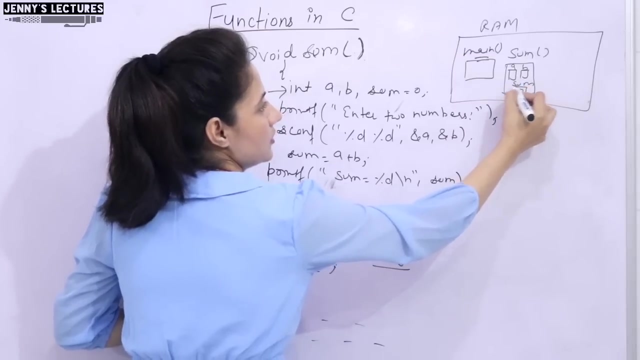 right. So memory has been reserved for this main. in main we are calling sum, right, So now sum is another function, right, and in sum, now I have a, b, So here we have a, here we have b, and one more variable, that is sum. sum is equal to 0. enter two number. suppose you are entering 5 and 6. 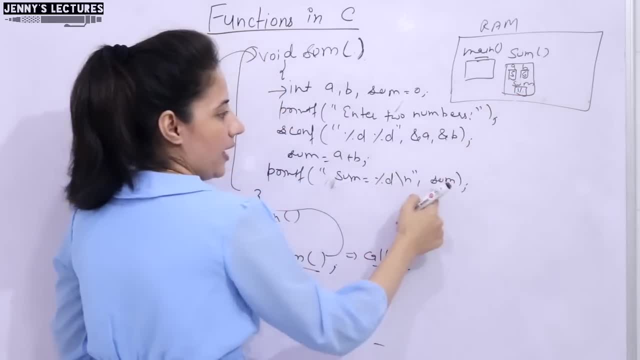 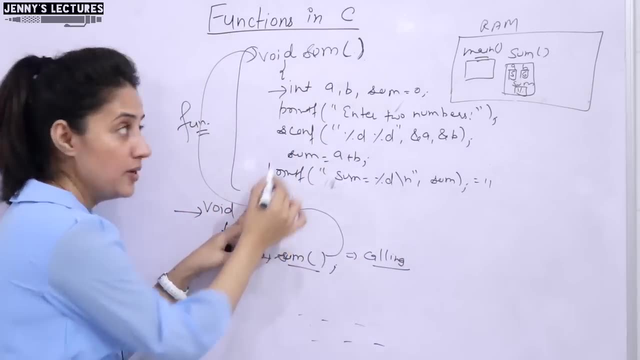 sum is equal to 0.. So here we have a, here we have b and one more variable, that is sum. sum is equal to 0. enter two, maybe several times, say 0 from b. This is one and a half percent of a, and we can say: 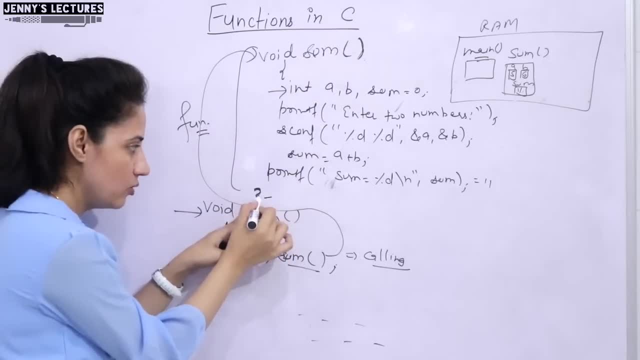 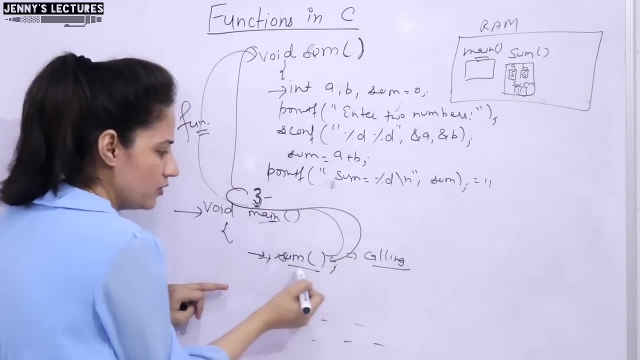 equal to 10, raise the limit point. So this like that. okay, if it is one reading from 0 reading plus b, then it is able to input 3 and 1 knit and then after finishing this block it goes to right and then you we can say that right. So yes, we use this idea that in the code of the order85. Sum is equal to a plus b, that is, in sum we have 11 and it would print 11 right now. after the completion of this nine, this is what, completion of this one. after completing this, as soon as you reach to this closing braces, control will go where back back to here, because obviously here we are calling sum right and one. when control will go back to the sum, then obviously we are going to pipe plus b and also we have 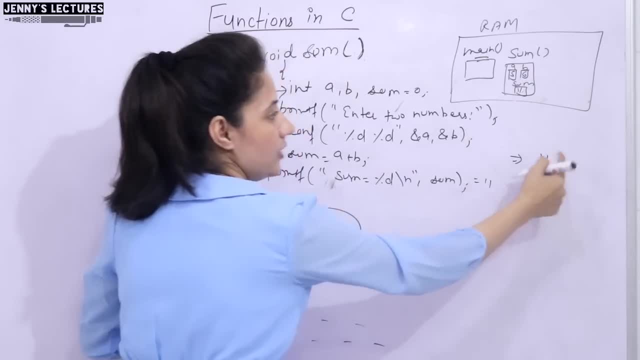 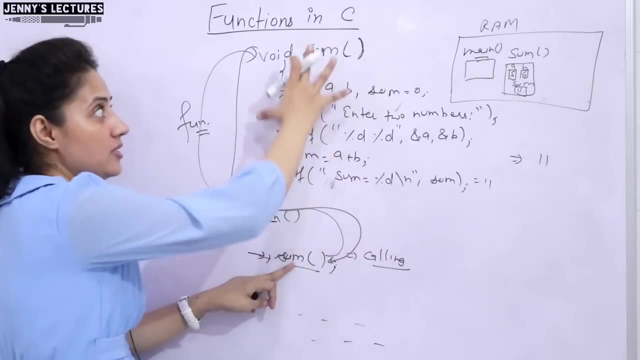 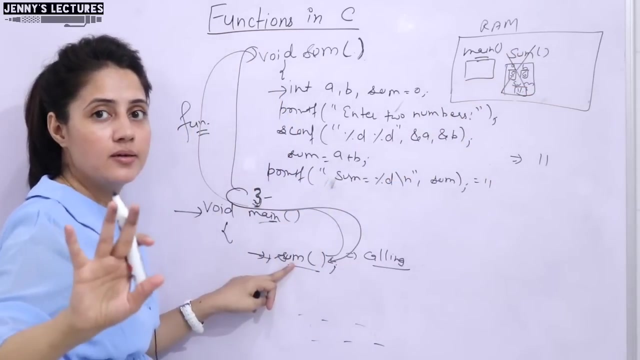 sum. then obviously on screen we have got 11, output screen we have got 11 because of this printf. once control will go out of this- here means out of this block- then this memory will be released, will be freed. right now, this is no more a reserved memory for this a, for this b, for this sum, because 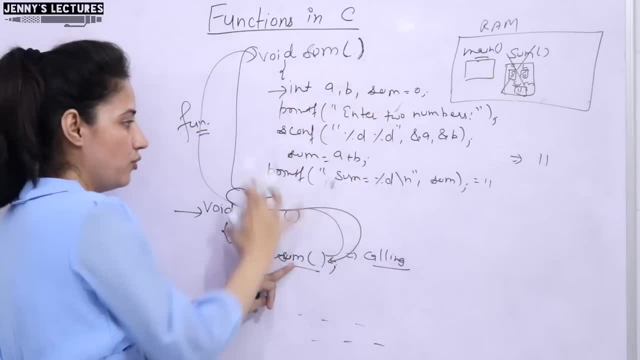 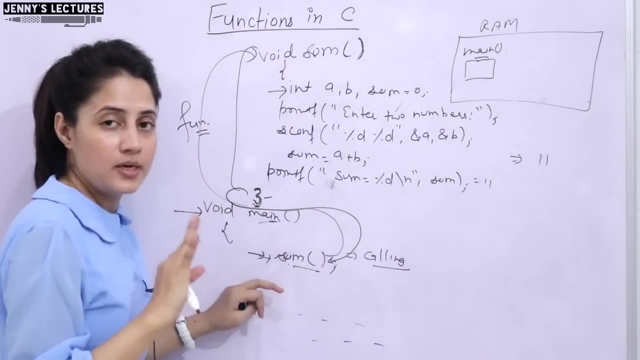 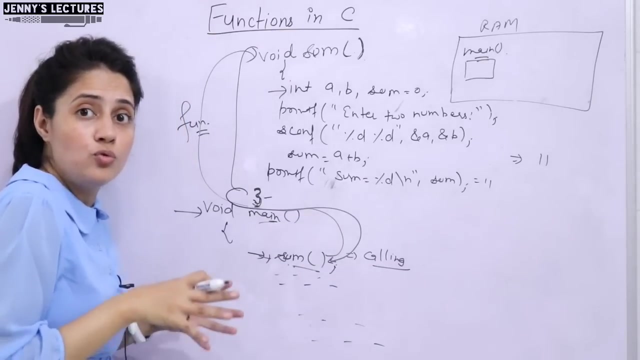 a, b and some. these are local variables, so whenever you go out of this thing, these, these would be vanished. so now this is free memory. we haven't reserved this memory. now, right now, again, suppose i have written some lines of code and again i want to do sum, so simply. 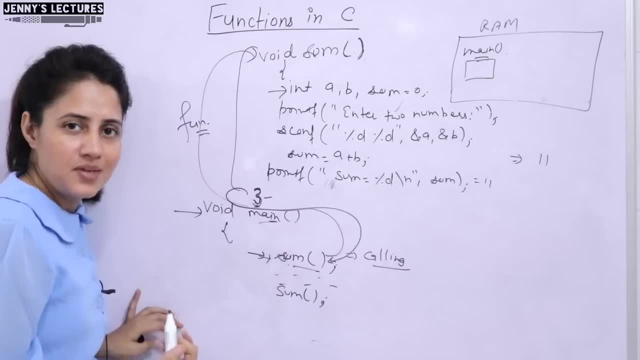 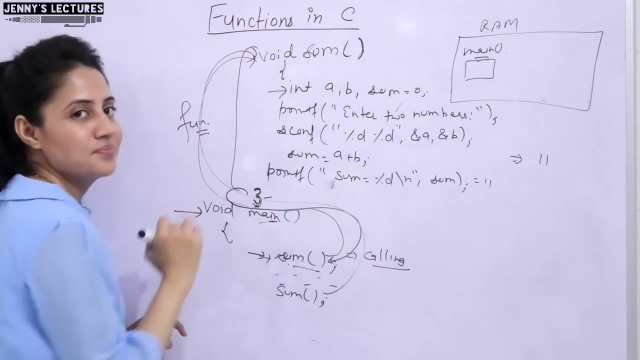 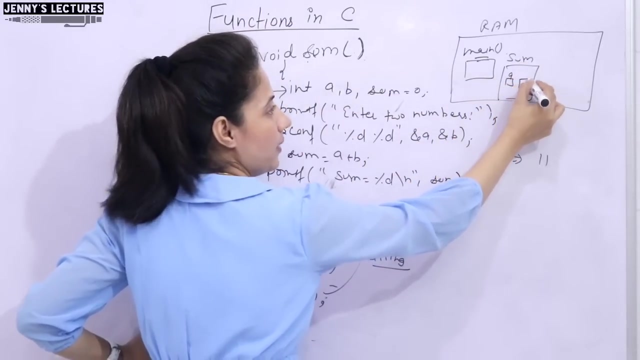 again you can call sum a single line you have to write down right and again. now control will go back to here. so now this would be loaded here in memory. sum you, because in sum we have a again. memory would be allocated to a, b and sum right again, suppose now. 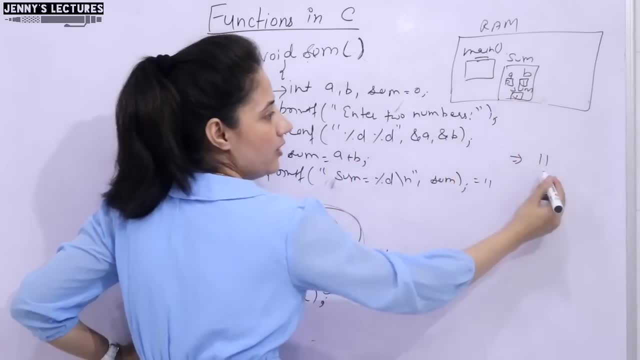 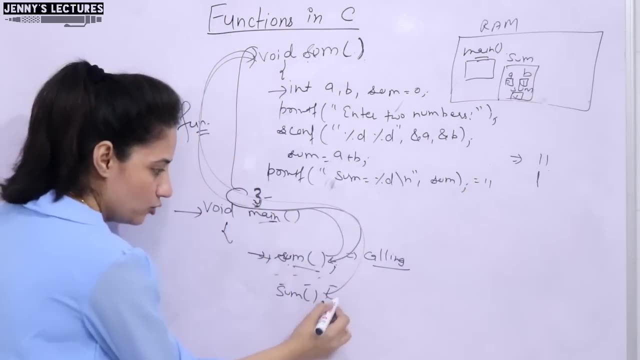 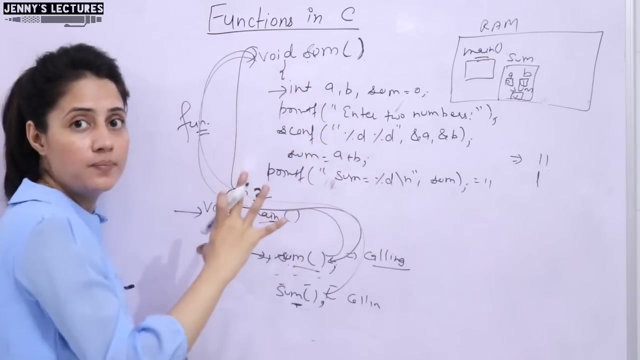 at this time we are entering 0 and 1, so now sum would be 1 and 1 would be printed on the screen. once control reach to here again, again, control will directly go back to here, because here we are calling this function. so this is what calling, this is also calling and this is what definition. 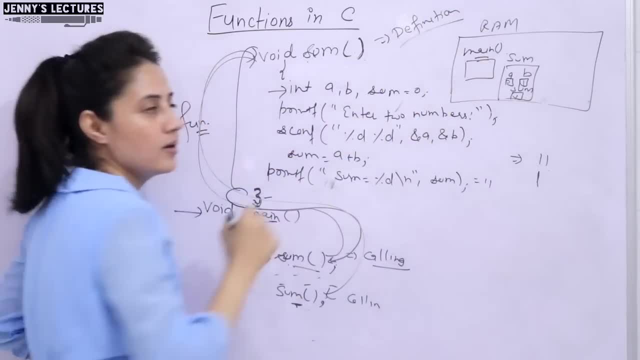 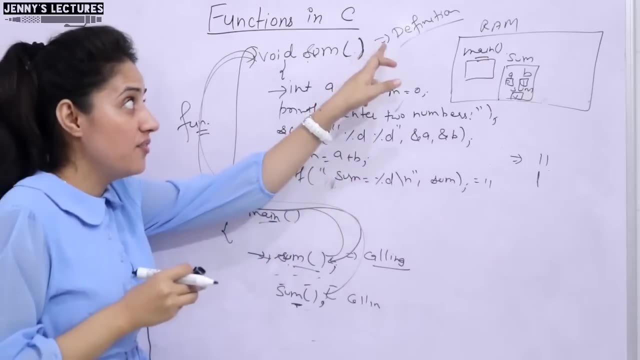 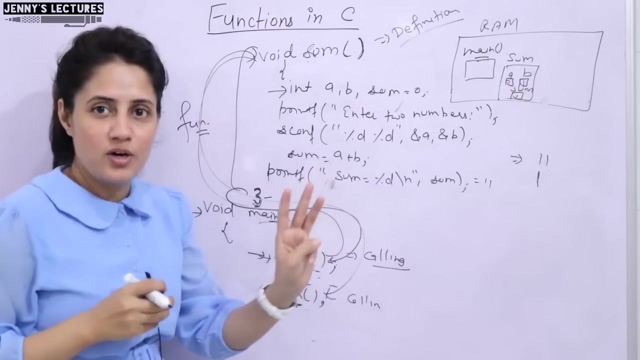 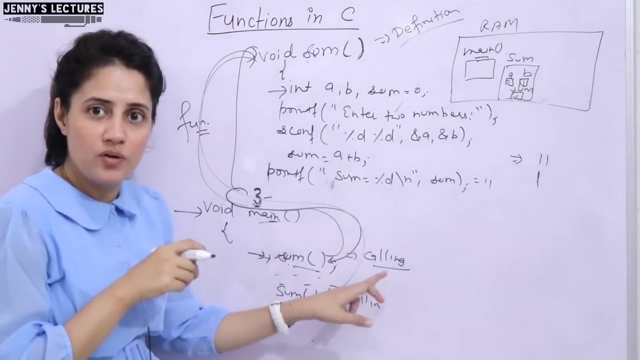 of function is, yeah, definition. we are defining what this function is doing. obviously we are defining this here. so this is definition of function, this is calling of function. one more thing: when we you know see function, three typical words are there with function: function declaration. or you can say: 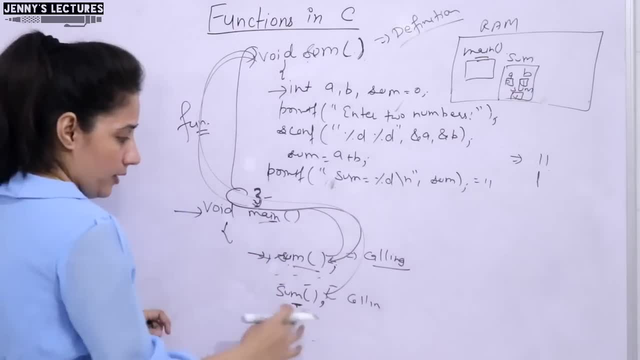 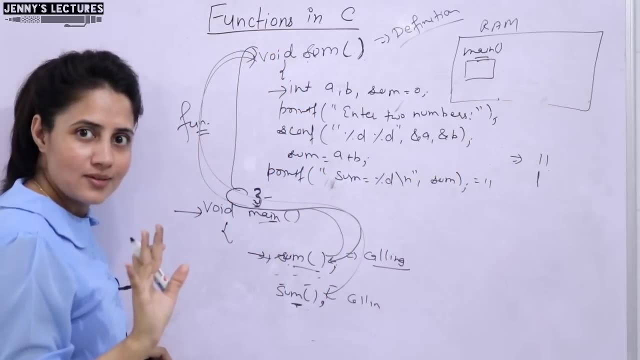 function prototype, function definition and function calling. so i hope we are clear with function Now control will go back to here. Now this memory would be released again. Right, Again, suppose. here, here I am. after this I am printing printf: hello. 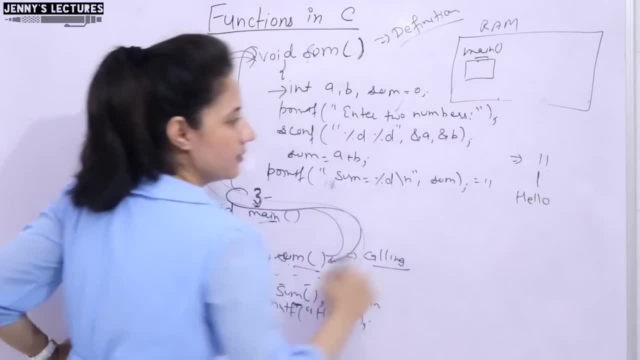 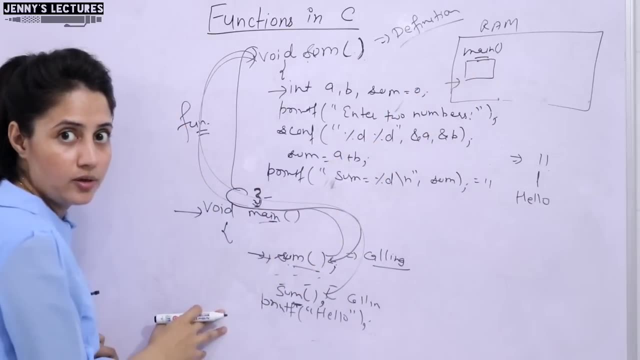 Right. So now at the screen word hello would be printed. Now main is executing Because we are now in main function again. Now main is executing Right Again after printing hello. suppose I want to do some again. 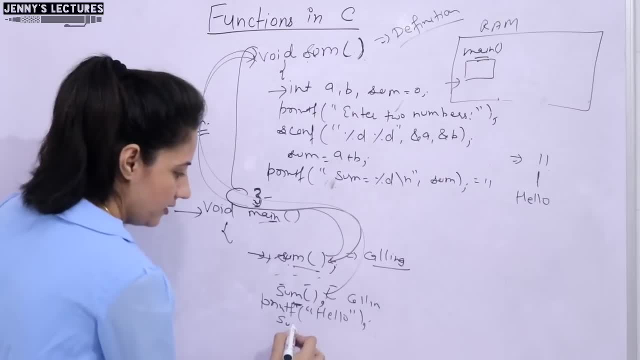 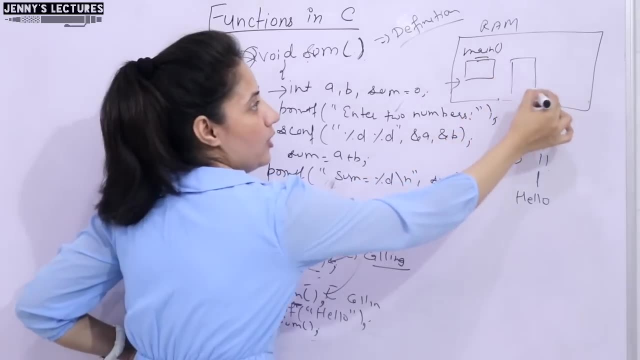 So again, you can call some. After this you can again write down. You have to write down just one line, Some Again. control will go here. Again, memory would be allocated to a, b and some. Suppose at this time you are entering number 5 and 5.. 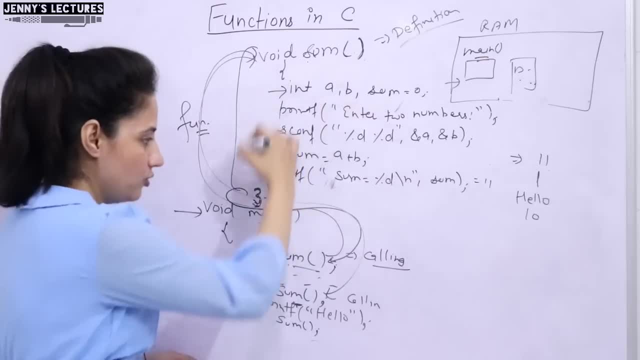 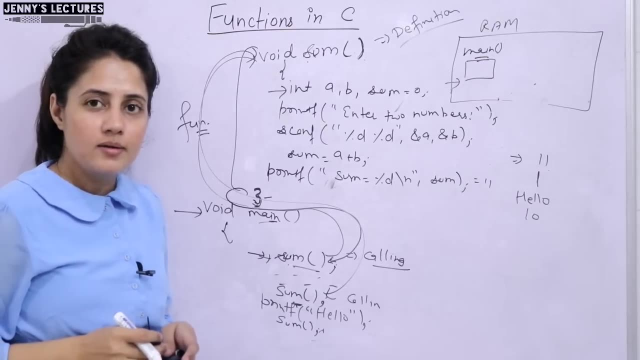 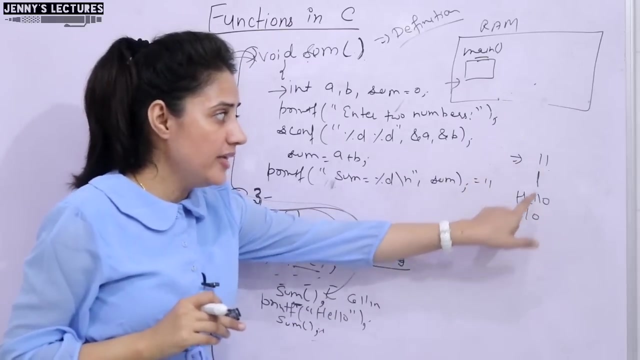 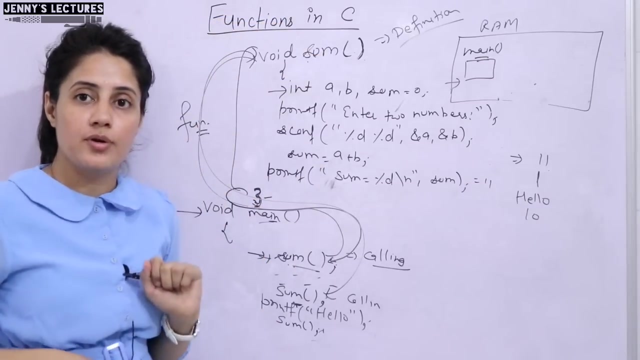 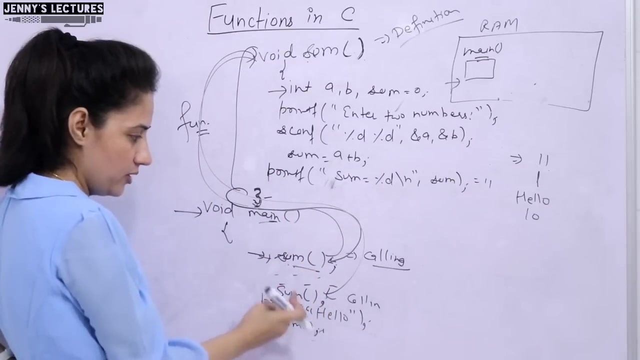 Some would be 10.. So 10 would be printed on the screen. After control will go back to here. memory would be released, Right? So I guess here I am. I am doing sum of two numbers three times, but you are writing the logic. you are writing this only one time in your program and whenever you, whenever you want to do sum, just call this one. just you have to write down a single line, sum, and the function like this: these, these bracket, that's it. 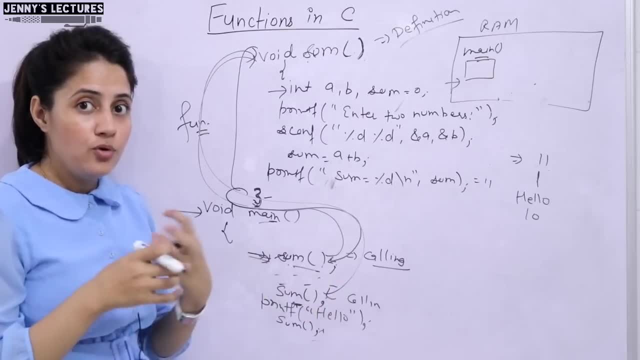 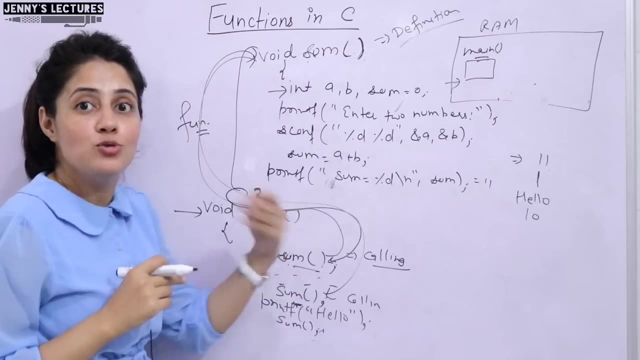 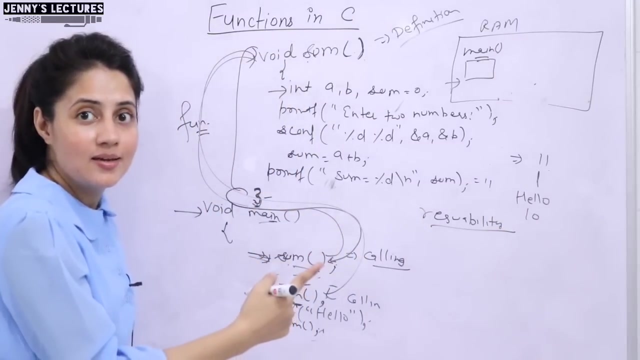 Right, Okay, So now I hope you got why we are using functions. So why we are using function It support? because reusability, How reusability. We are using this code again and again in a program without writing it again and again. 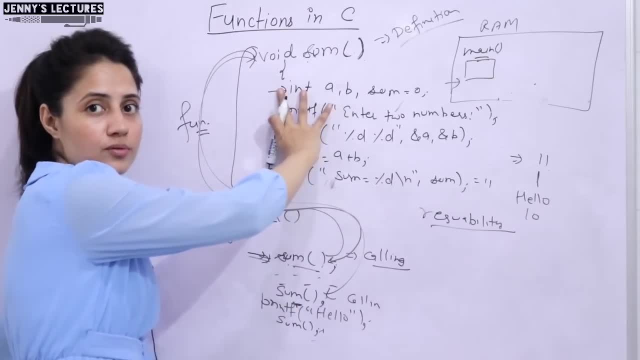 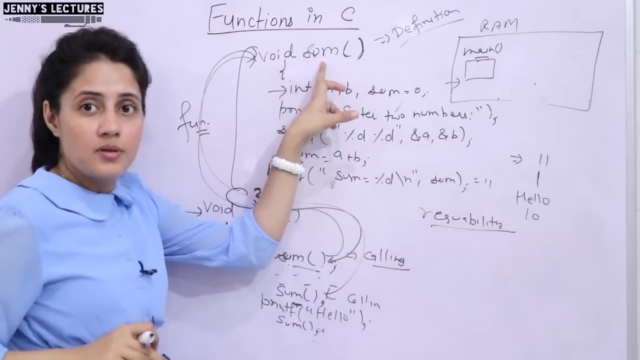 Some, some, some three times. we are using this code Right, Right And it's. It's just a single task. there can be multiple thing like sum in a program, same program I am calculating number is prime or not. 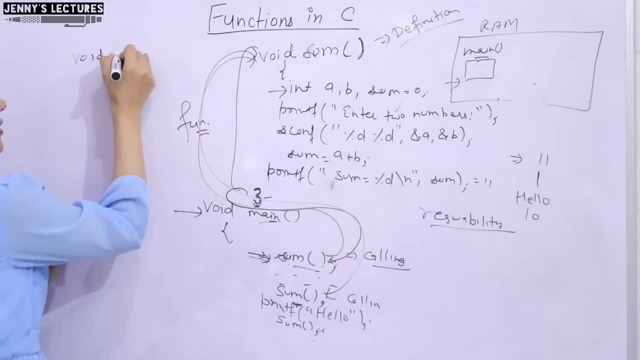 So one function you can write down here: void is prime and here you can write down the logic, like number is prime or not. here you can write down the logic and here you can call that function if you want to call. 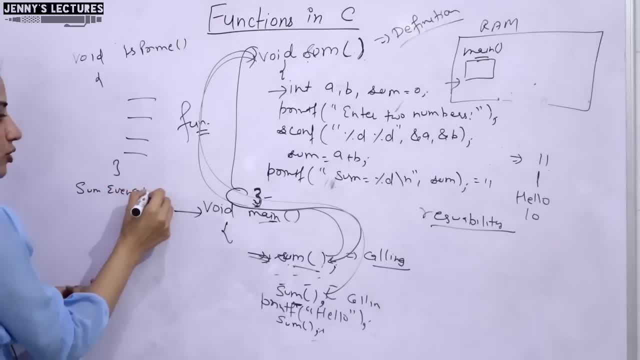 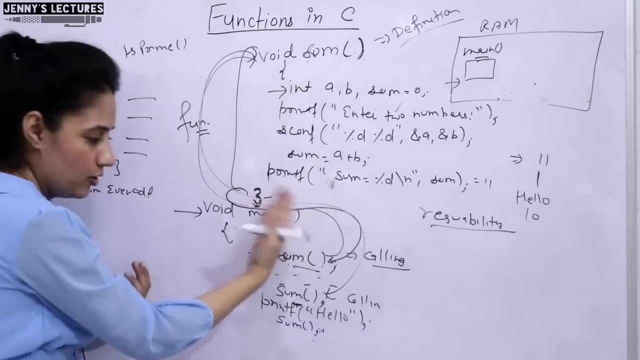 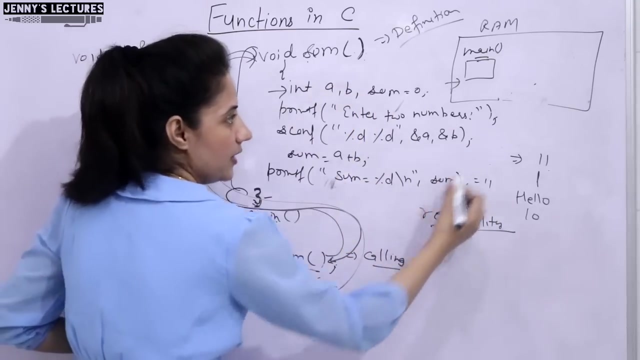 One more function. maybe you can say even or odd. So one more function. you can write down something like this: you can define that function right, Write down the code and you can call that function in sum. So suppose I am calling 5 times sum, right? 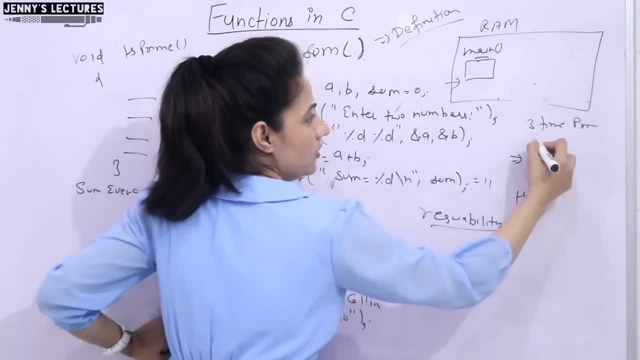 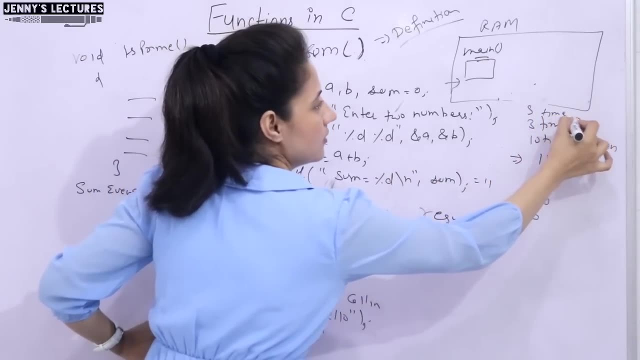 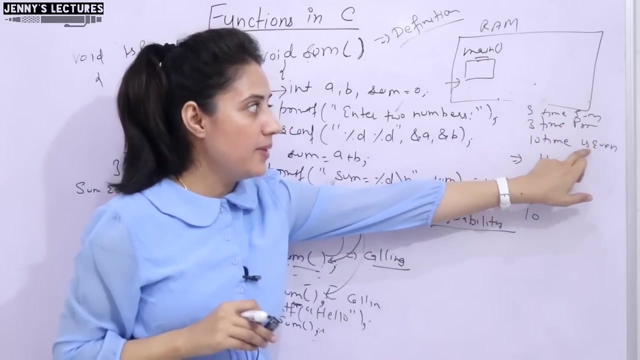 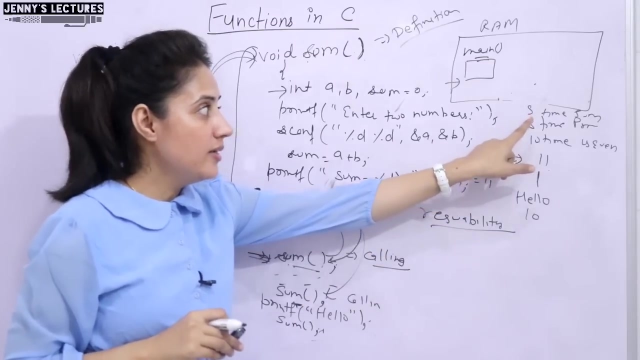 3 times that prime function and 10 times even or odd and 5 times sum. Right, So 3 functions. Then we will create: sum is prime and is even. Only one time you have to write down the logic, the definition and you can call it 5 times sum here. 3 times that is prime function and 10 times is even function. 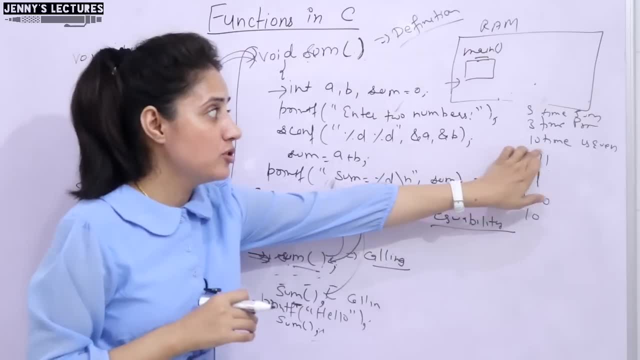 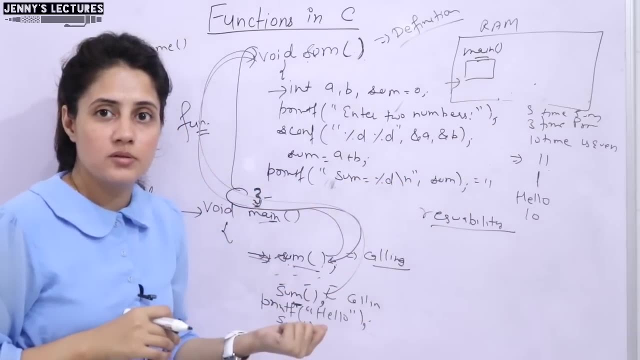 You don't need to write down the logic again and again, like 10 times logic for is even 10 times logic for checking number is prime or not? 5 times logic for doing sum of 2 numbers Right? So here we are reusing these function again. 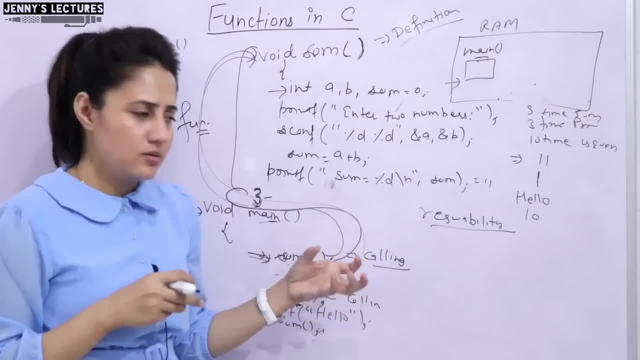 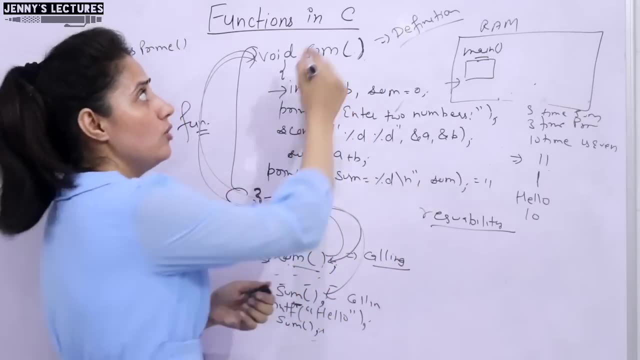 Again and again. So this is what reusability. So this is a very basic level right. Generally, when you write down you know these are also code. you can say function or module Right Or sub program. 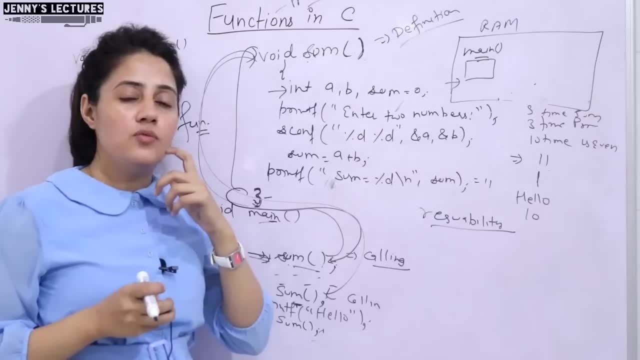 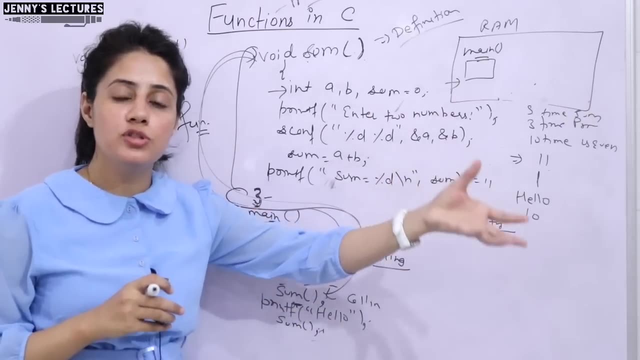 The same thing, right So same. when we are going to build a large project, when we are working on a large project, then simple, simple, reusable modules are there. You can directly, You know, use those modules in your projects. 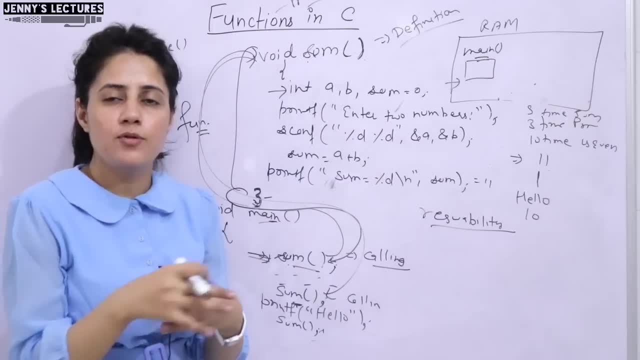 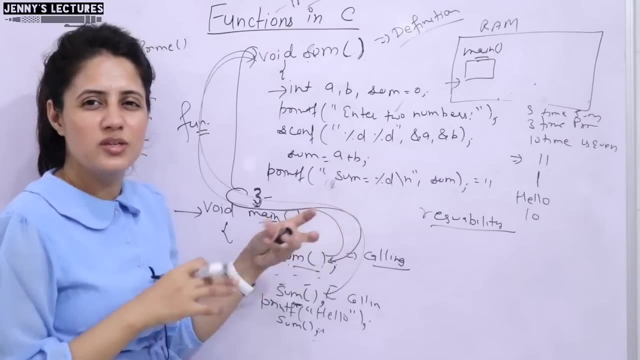 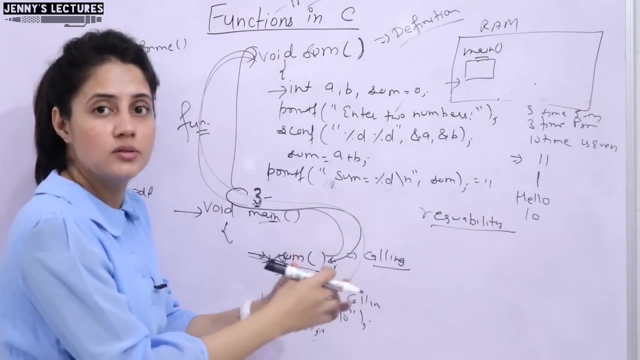 You don't have to write down the coding again and again, Right? That would be a very- you know at that level, high level. This is basic level. I'm just explaining function using a simple example, Very basic level. Whenever we will go deep down in the function, then I'll show you, then I'll tell you the actual why we use functions in industries also, like in projects. 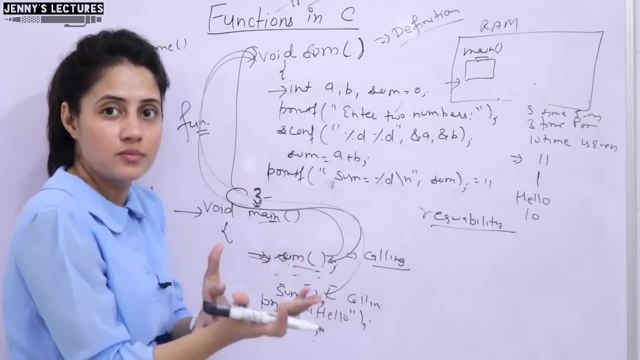 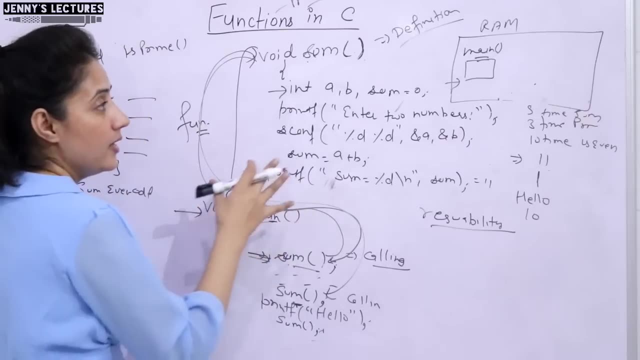 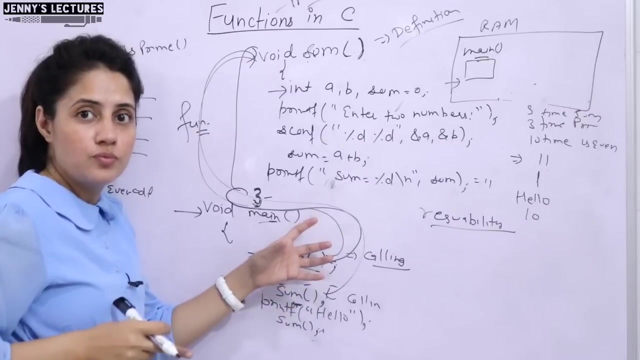 When we are developing softwares there, that would be really very beneficial to use functions or you can say modules, right? So now I hope this is clear. Second is what if you use functions? first is reusability, second is what: it's easy to test the program or debug the program right. 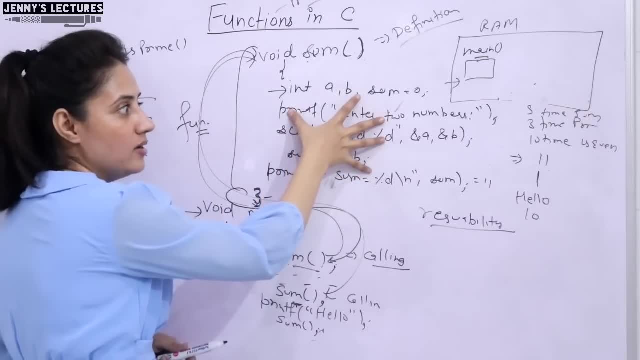 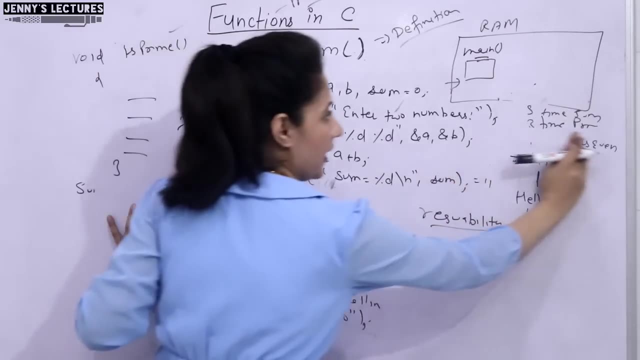 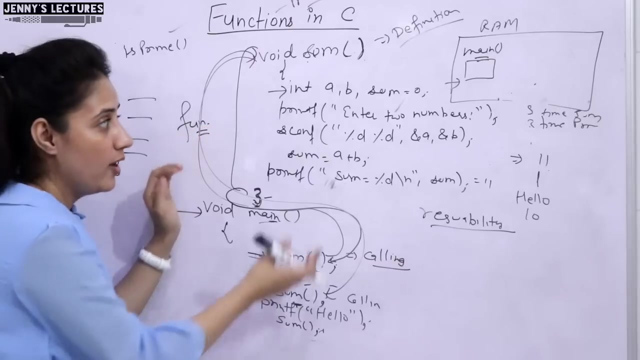 So simply, here I'm writing one module, one function for add, one function for suppose is prime two function. I'm taking And I'm copying, I'm calling here five times sum and three times this function. Now the program is small length line of code. is you know less here? because you are defining the sum only one time rather than five times. you are writing these codes. 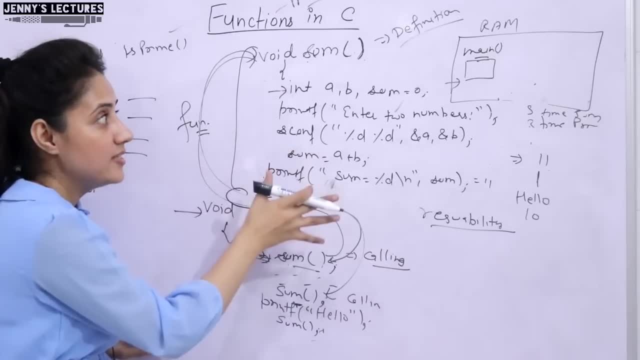 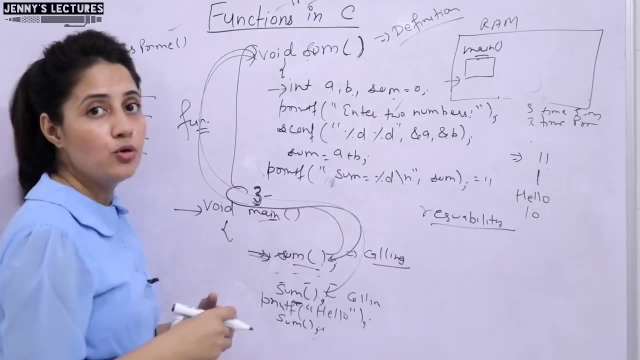 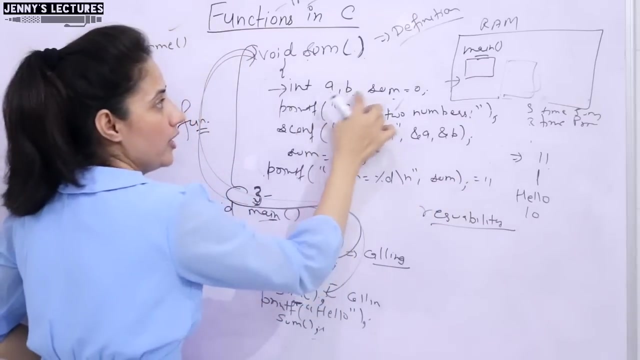 So debugging is also becomes easy. Next is what? if you use function, then it would be memory, better memory utilization. How better memory utilization? See here I have told you the working. Whenever control will go off, Go here, then only the memory would be allocated to A, B and sum to this, sum function. 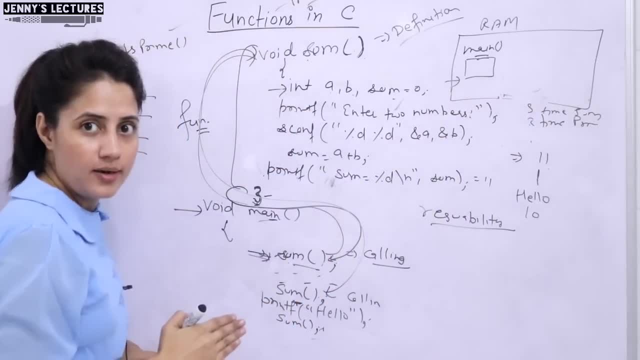 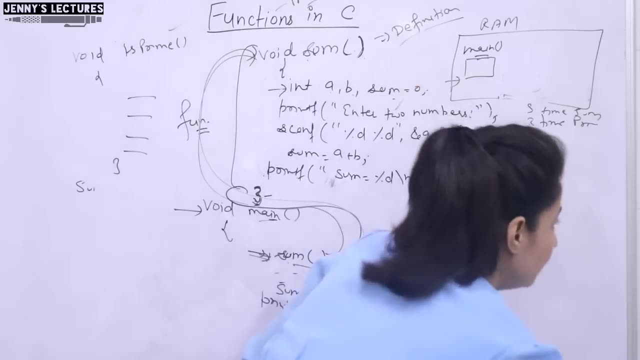 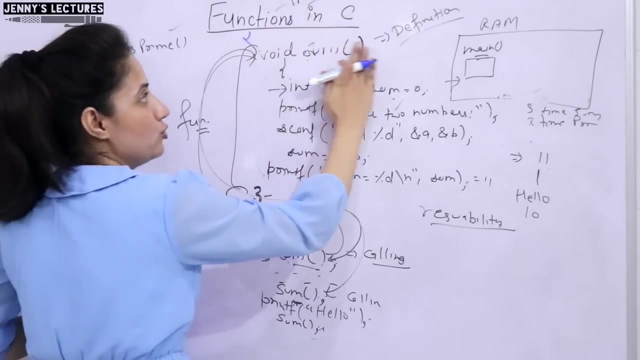 Once control will go out, this memory would be released. right, It's free, You can use this memory for any other purpose. Operating system will use this memory for any other purpose. But suppose if you write down this in main function, suppose here only I'm writing main and I'm not using this function. 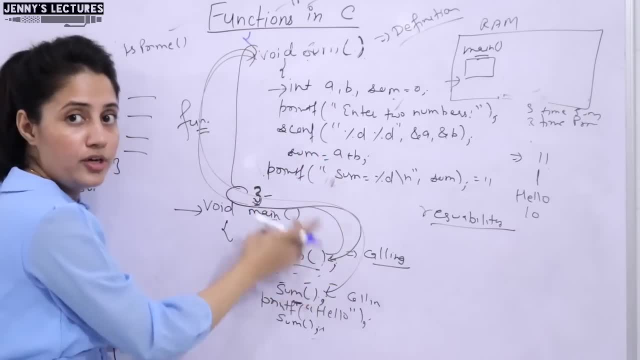 I'm writing the code in main function maybe five times, or in main also I'm doing any other thing also, Right? Rather than doing some some other thing also I'm doing, right? So these scope of these variable would be throughout the program, till end of the main function. 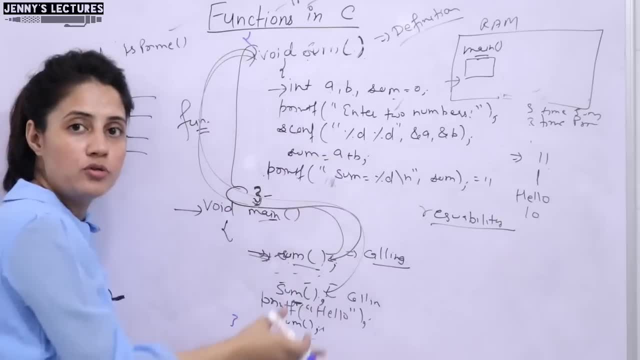 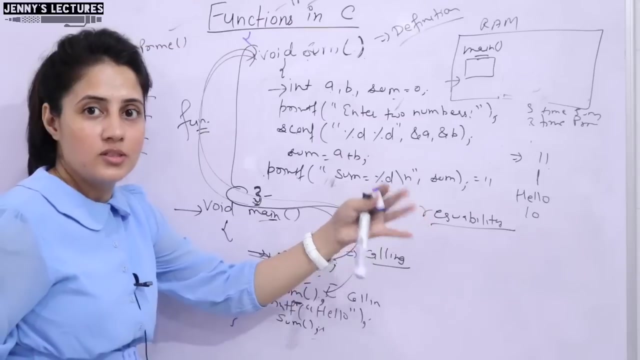 So these variables would would hold the memory throughout the program, right. But we don't want this thing right, So better to use function, So that will be memory, that will be wastage of memory. So if suppose your program is very lengthy, very long sometimes, Because sometimes it it is not able to find out space for your program. So that is not. you are not able to execute your program because of small memory, right? So better to use function. So that would be better memory utilization. 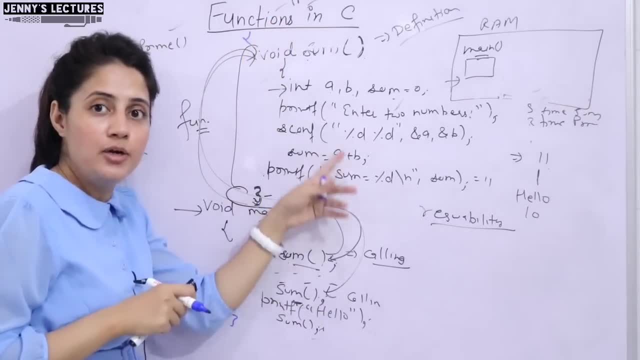 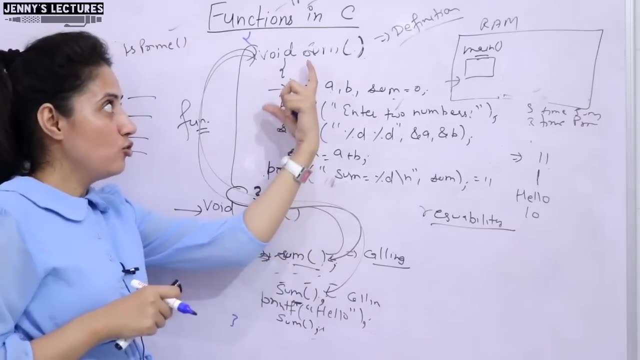 And if your program is still very lengthy, but still you are able to execute your program in the memory because you are using functions. So whenever control will go to this function, then only memory would be allocated to this Once control will go out. 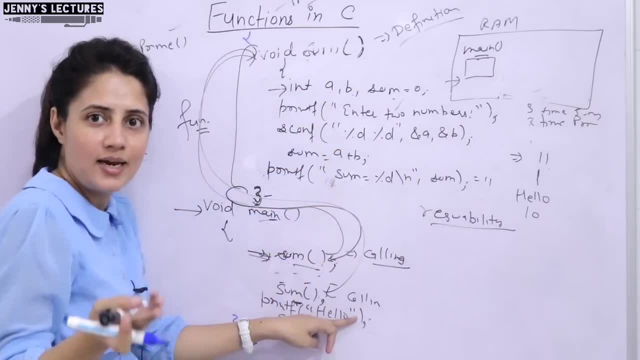 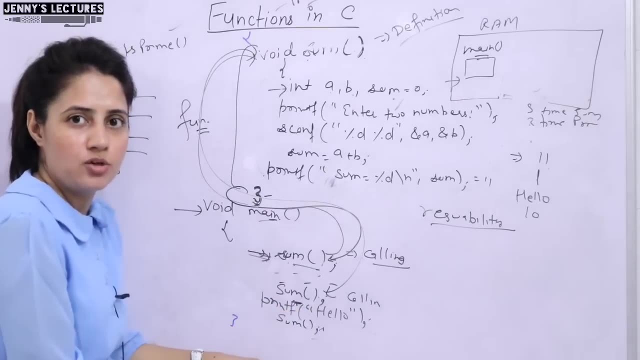 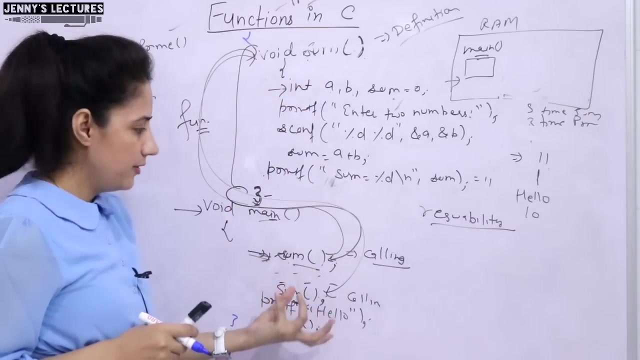 To the main function, memory would be released. That's it. And in main function, if you are writing some other code, maybe some other code, you are doing some other thing also, Then that would be executed right. And also one more thing: you can say: function: if you will use, then it will also. definitely it reduces the complexity of the program. 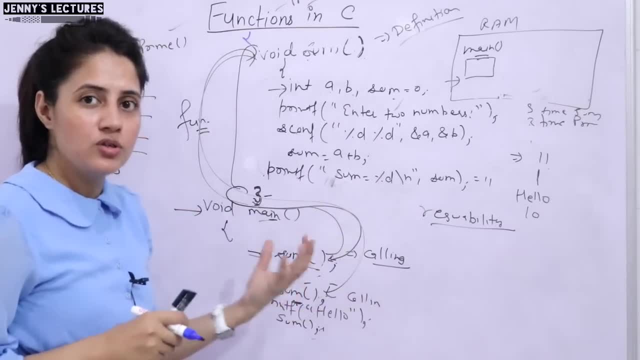 So these 3 to 4 main you can say reason why we are using function, Or you can say these are advantages of using function. So I hope now it's clear to you why we use function. So I hope now it's clear to you why we use function. 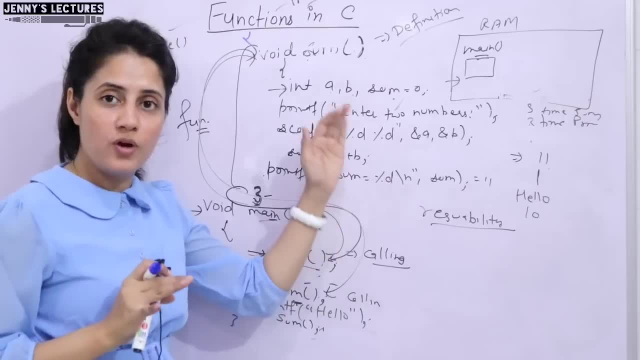 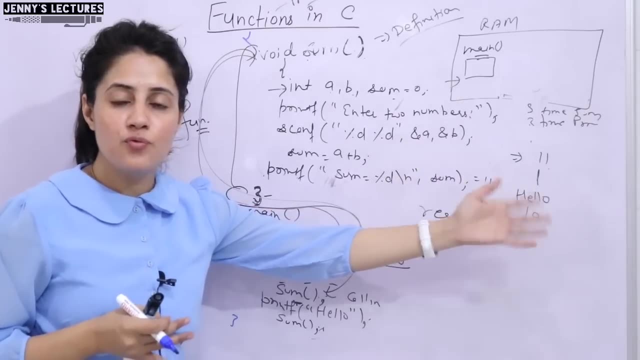 So I hope now it's clear to you why we use function. So it's always a good practice to use function in your program rather than writing the code- all the code- in main function. Till now we have discussed programs where I was writing code in main function only. 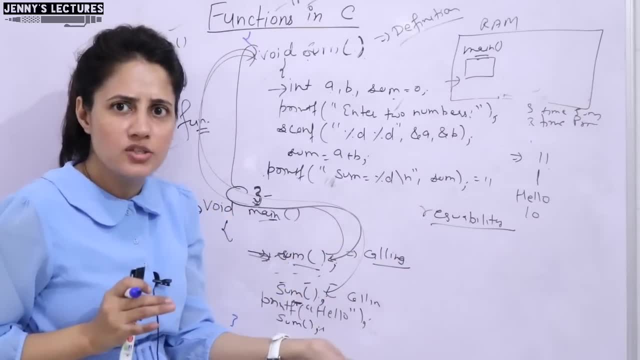 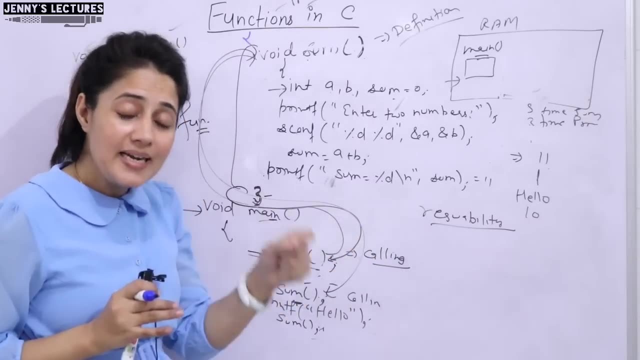 I was not using any other function, user defined function. Main is also a function, right, But that is what. obviously program at least this is also very important. A program must have at least one function, that is main function. 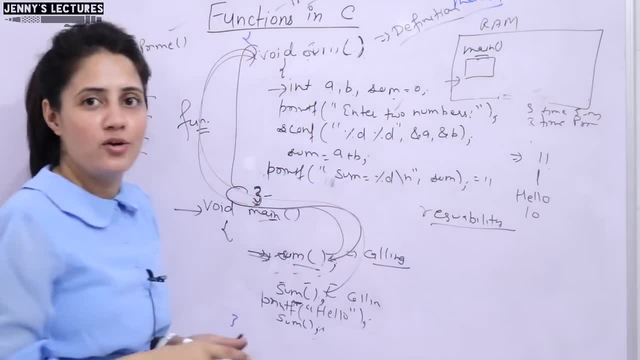 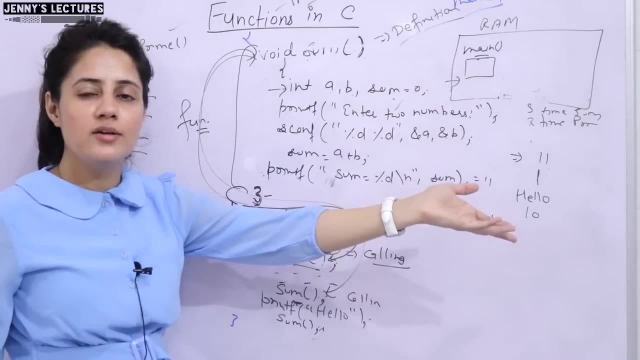 A program must have at least one function, that is main function, Because obviously without main function you cannot run your program. So at least one function must be there in your program: main function. Other than that you can use any function, any. these are what you can say. this is what user defined function. 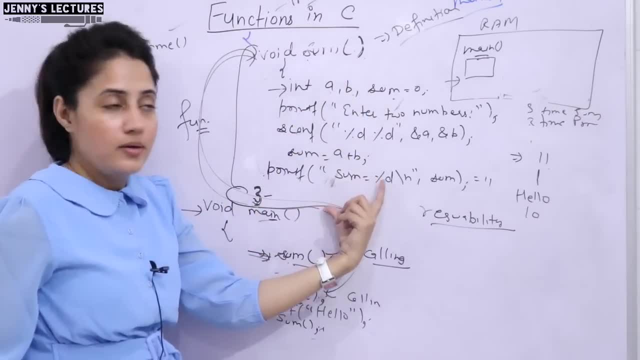 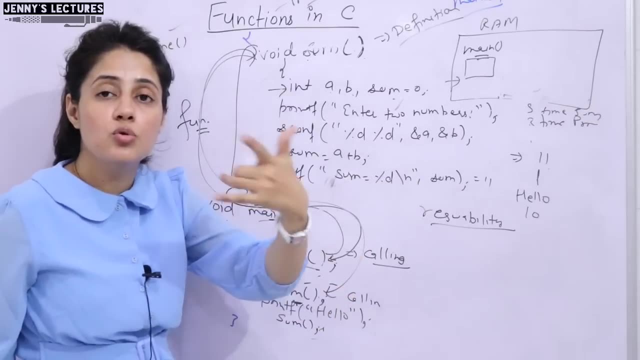 Because we are defining this function. we are writing the logic here. Is prime, this is also user defined function. we are writing the logic here. Printer scanner, these are also function, but those are predefined function, library functions Already defined in header files, right? 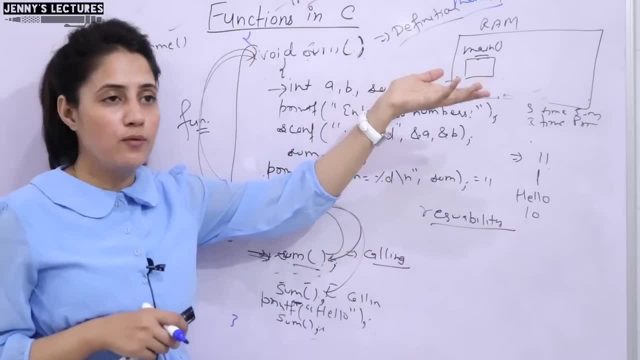 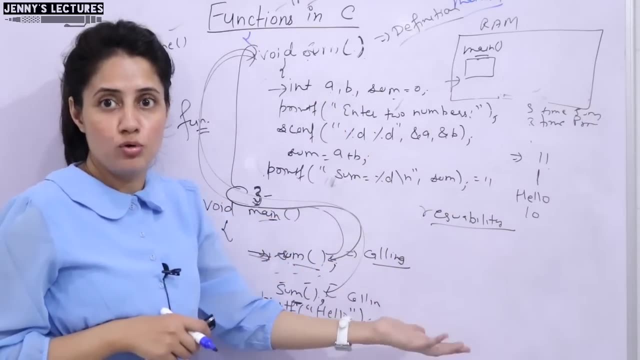 Meaning of those functions already defined in header files. We do not have to tell the compiler meaning of printer, meaning of scanner, Meaning of clear screen, meaning of get ch right. Those are also function. we are using predefined function in program, in our program, right. 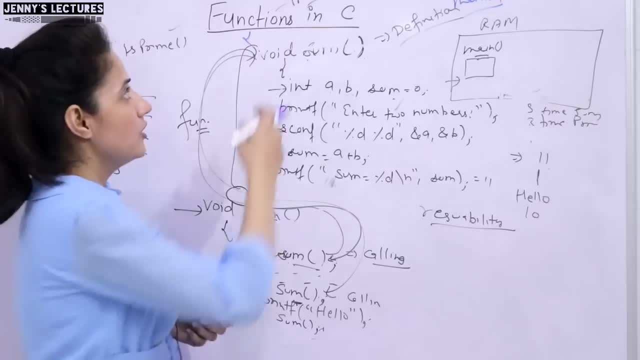 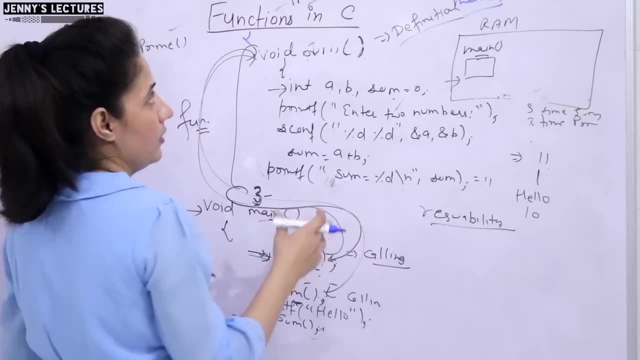 So I guess this is clear to you why we use functions in C, Or these are also called modules. So that is why C is also known as modular support. C supports modular programming. So if I ask you, what is definition of a function? function is what. 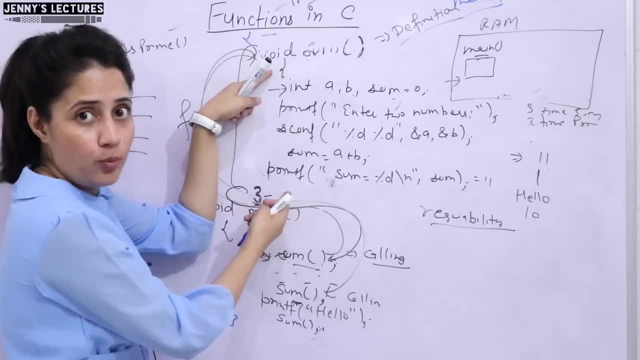 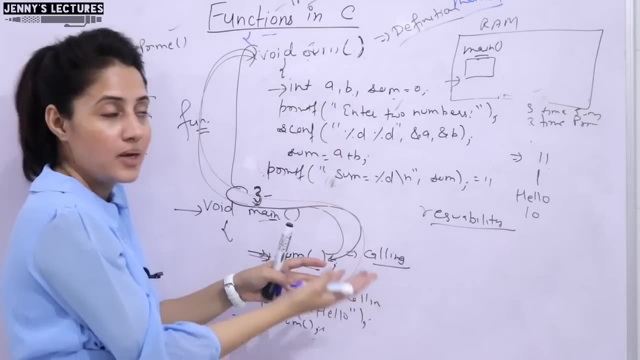 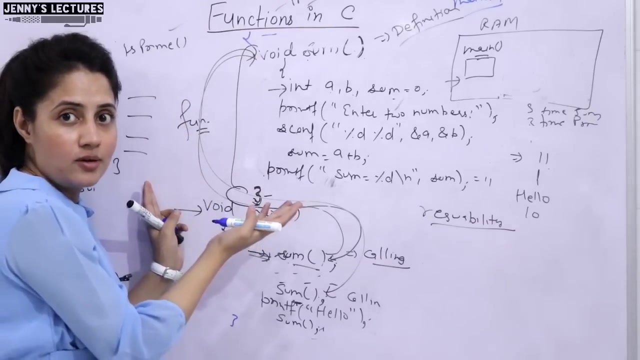 It is a piece of code. obviously it is a piece of code, or you can say group of statements, that perform some specific task. This perform is this function is performing. some is prime. This function is also performing a specific task. checking number is prime or not, right? 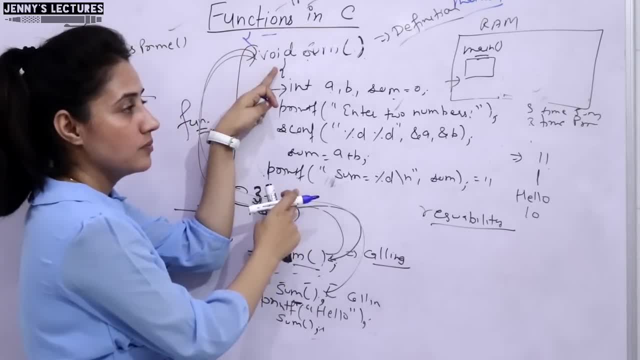 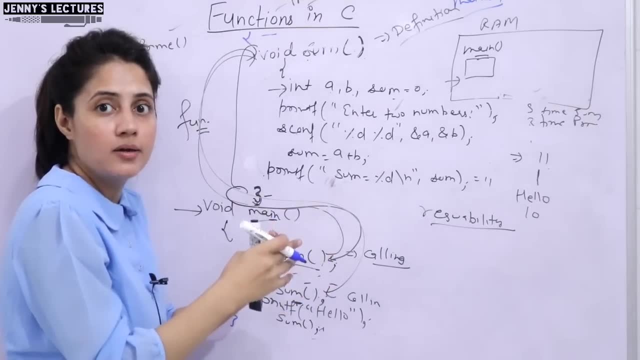 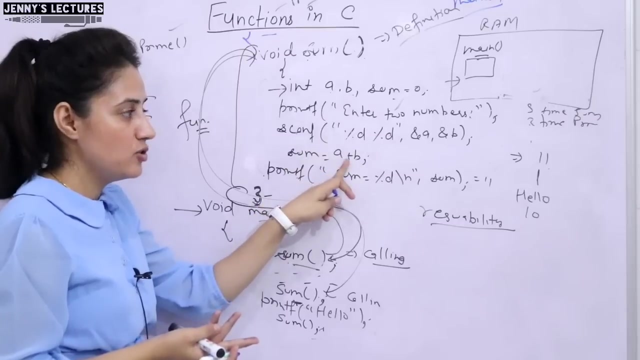 Or you can say function is a piece of code which takes some input. So this is the definition of function. So to prove that we have to do some computation, some processing on those inputs and gives you output. Same thing this function is doing. 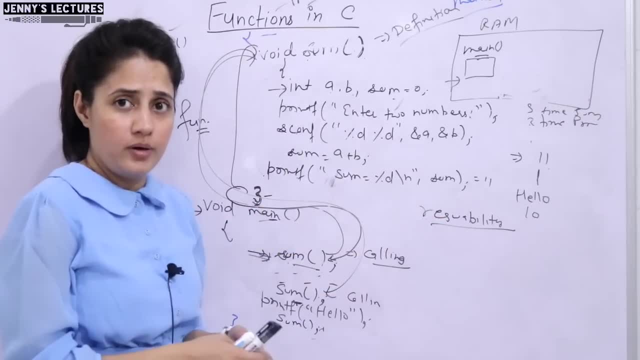 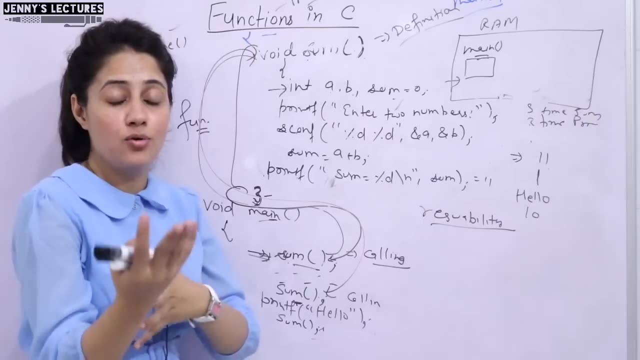 Like it is, taking input, processing sum is equal to a plus b- and giving you some output. So I hope you are clear with the definition and why we use functions So you can write down your own definition in your own language: the definition of function right. 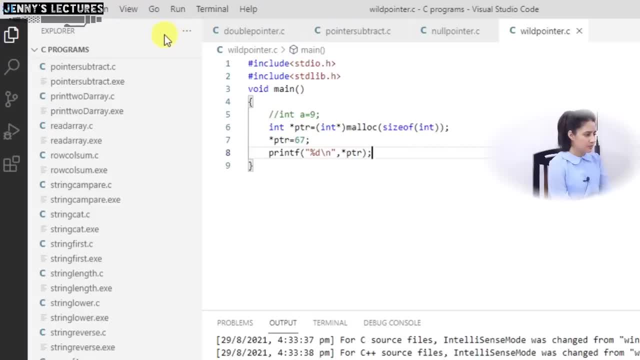 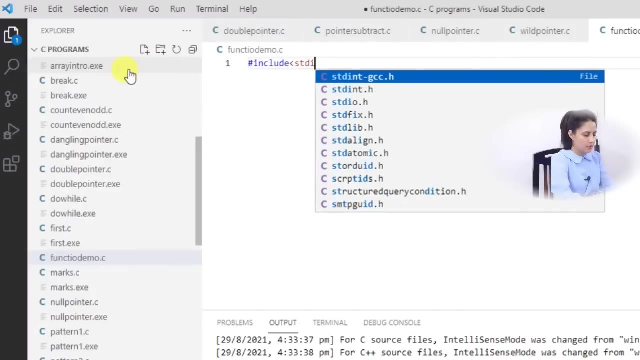 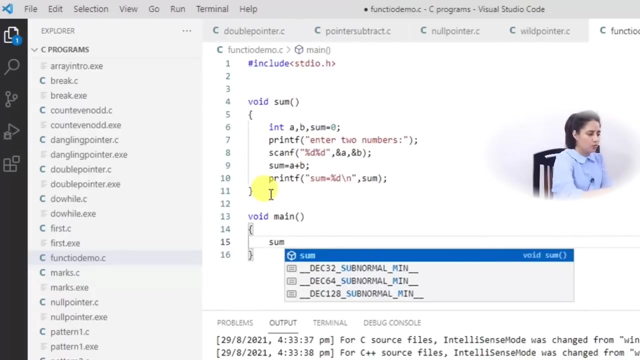 So now let me show you practically. Now let me create a file, function democ. I am writing the name this, and here I am using what? here I am defining this function sum right. And now in main function I am calling this function sum here right one time and then 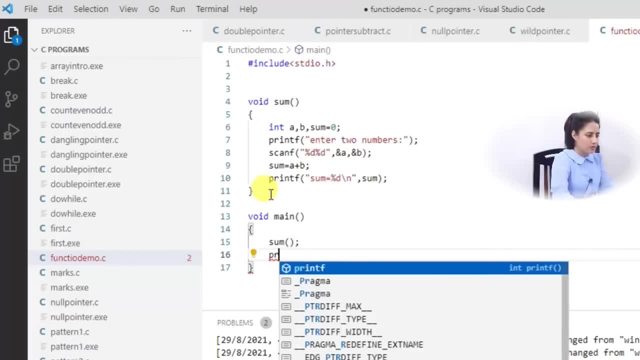 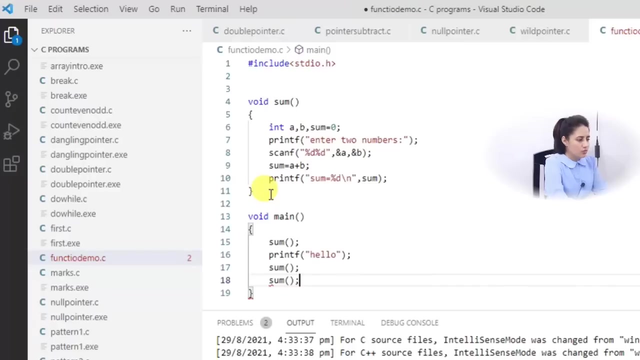 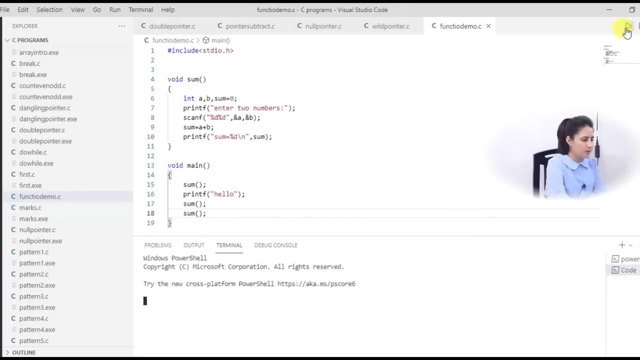 suppose I am printing hello, And after this again I am calling sum- right, And now again I am calling sum three times right. So let me run this and see what output you are getting. First of all it should ask like enter two numbers, because first we are calling sum first. 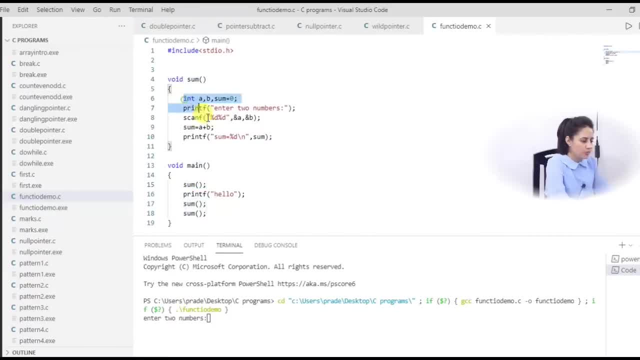 So it will go to the definition part and it will ask two numbers. enter two numbers, 4 and 5.. So see, sum is 9. it is printing now. next line is control will go back to the main function. now next line. in next line it will print hello. 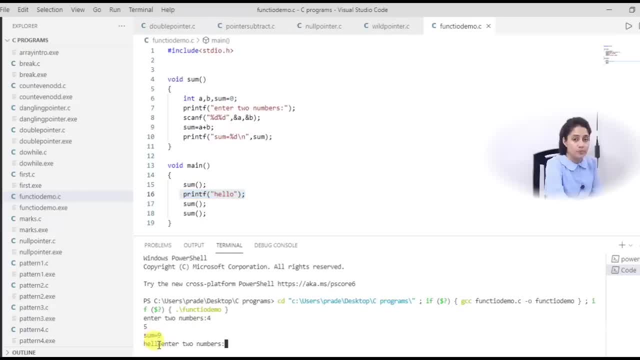 So it is printing hello. again we are calling sum means: again control will go to this definition of this main function, this sum function, and again it will ask: enter two numbers. So I am entering here 5 and 6.. So it is giving sum 11. again I am calling sum. 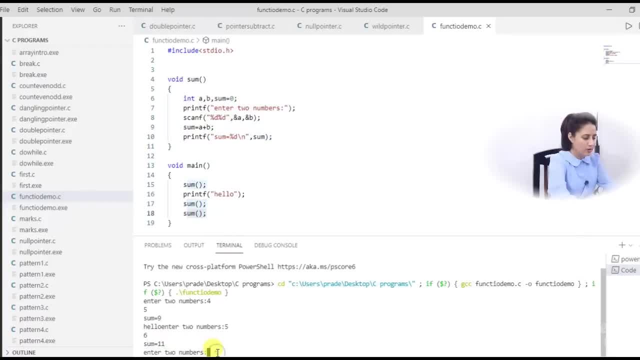 So again it is asking: enter two numbers. so this time I am entering 1 and 2.. So now it is giving: sum is equal to 3, right? So three times I am calling this one and I am writing the definition part only one time. 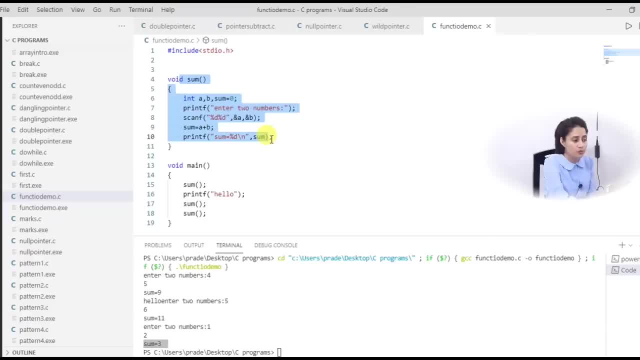 right, not three time in my program, right. So this is beauty of using function and in main also main: you can also do some other thing rather than just calling some function. or maybe you can use more function also, like subtraction, multiplication, Those functions you can do. 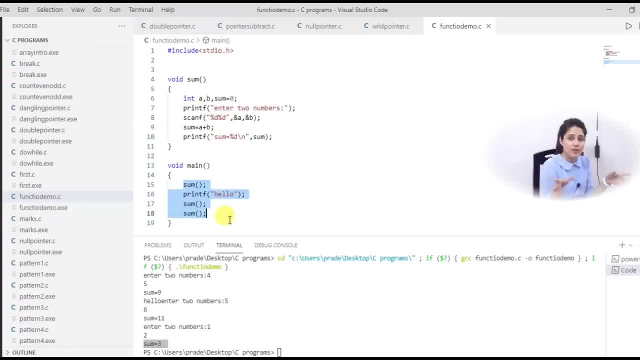 Those functions you can call in main multiple times. So you can call a function multiple times, many times, and it is not necessary that you will always call a function in main function, In sum function. I can also call another function. maybe suppose one function is subtraction. 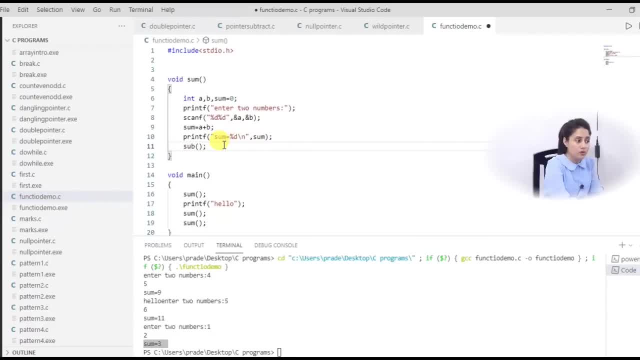 that I am going to call here right. But first of all, obviously we will write down the definition of this subtraction sub. So here in these curly bracket, You can write down the code of, you know, subtracting two numbers. This is also fine. 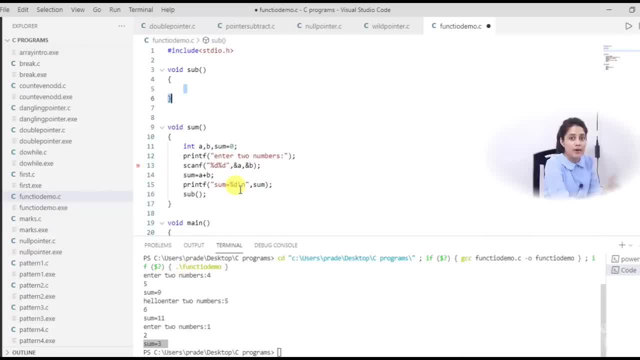 You can call a function in any other function, but you cannot define a function within other function Here. in sum, if you want to write down definition of subtraction like void sub, and here you want to write down the code of subtraction, this would be illegal. This is not allowed.